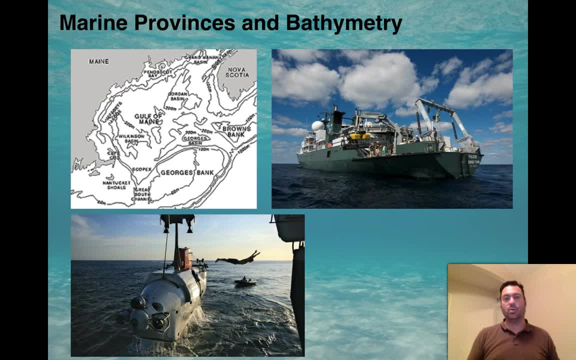 you know, into the depths. in that sense, Looking down into the water, almost like a bath, Cool. So let's go ahead and jump right on in A couple of cool pictures. here We'll be seeing some of these things. This is a bathymetric map. This is Maine. 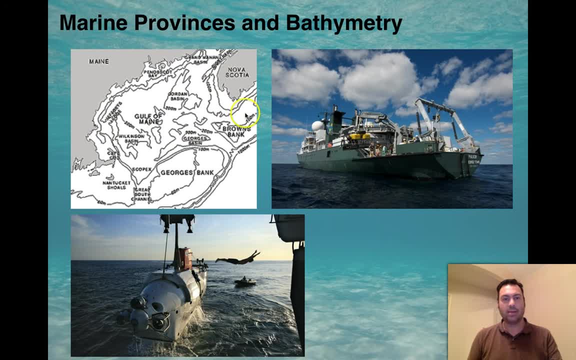 right here We can actually see that the sea floor off the coast of Maine has some interesting features happening out over here. Here's a basin, Here's a gulf. We'll be looking at how we know about this stuff shortly. Here we see a. 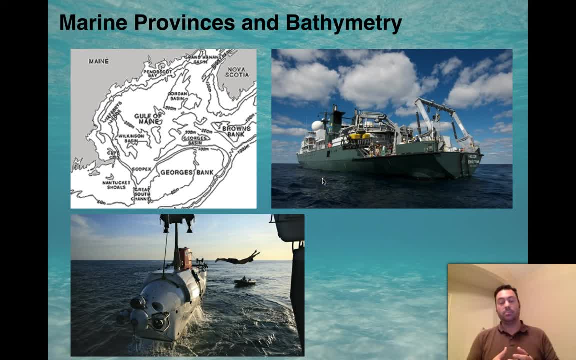 research vessel that has the ability to deploy sonar, and special submarines that have the ability to go out into the deep water and get measurements that they can get after they've come out of there. So it's a great place to look at these things and even photographs of the sea floor, and give us an idea of what's. 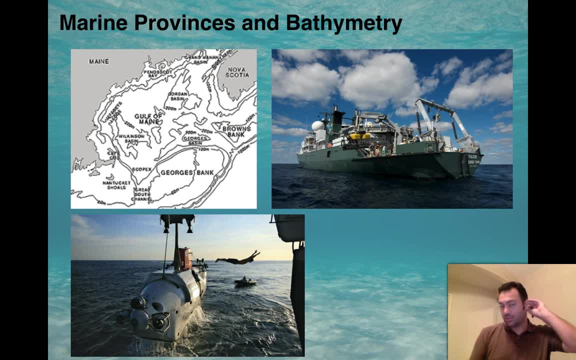 going on there and, of course, one of these really deepwater submersibles and somebody having a good time jumping off right as they're servicing the submarine in the same picture. All right, So we get an idea of what we're going to be talking. 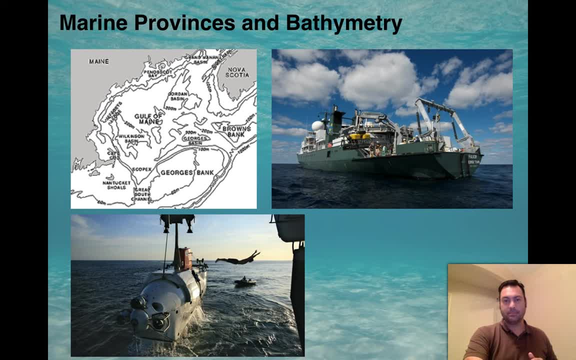 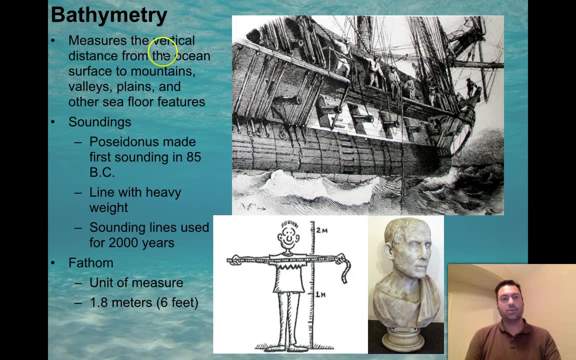 about today. This is where we're going to really start jumping into oceanography. As opposed to looking at the earth and all the plate tectonics, we're going to be looking measurements of the ocean right, So it measures the vertical distance from the. 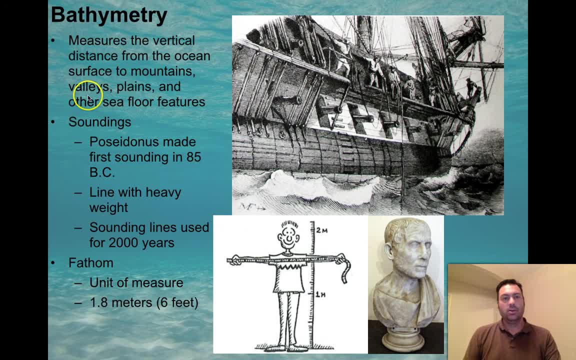 ocean surface, in other words, from the top of the water to mountains, valleys, plains and other seafloor features, right. So it does turn out that when we go down to the bottom of the water, as we described just momentarily, that there are 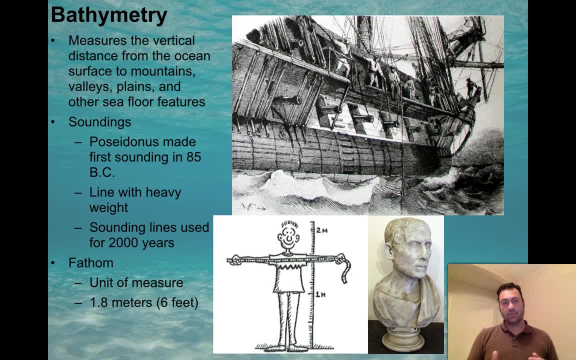 basins, but there's also mountains down at the bottom of the seafloor And what we would do is a process called sounding. A guy named Poseidonus made the first soundings in 85 BC, and what he would just do is drop a line. you know a rope. 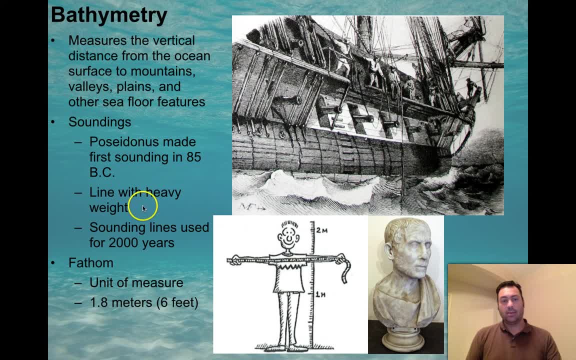 with a heavy weight like usually a piece of lead, And this is basically how we did mapping of the seafloor for 2,000 years, And the standard measure of depth is something called the fathom. So the fathom is down here. I lost my stylus. 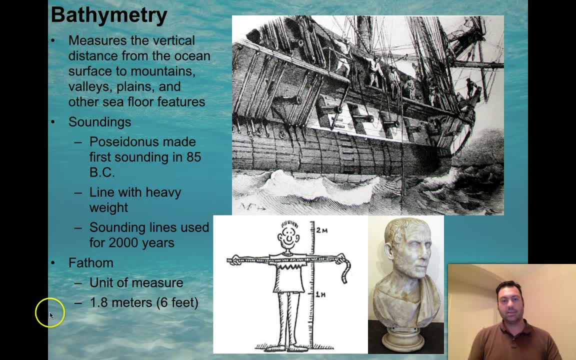 Yeah, here it is. So here's the fathom: It's six feet. So you can see it's six feet. So you can see it's six feet. So you can see it's six feet. So you might be asking: where does this come from? Well, look at this picture over here. 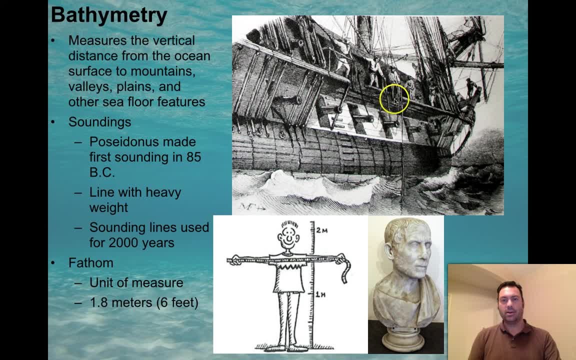 This is a really neat picture here of people doing off of the side of a British battleship soundings. They're dropping this rope down into the water and every time this sailor pulls the rope he would pull it the length of his arms. 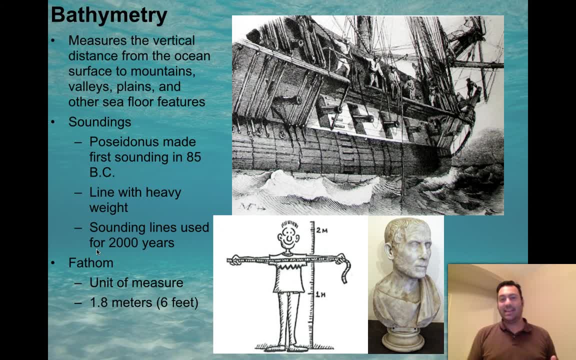 right, He'd pull it like so, And every time he did this that would be six feet, And if he knew, every time he pulled the rope, that would tell him how many fathoms You. multiply it by six, that would give you the number of feet for the depth, And that's a tradition that is still in. 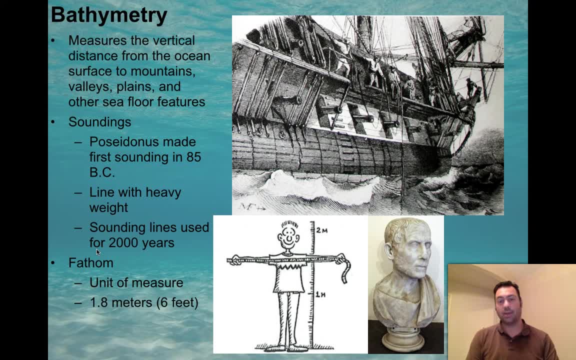 use today. You go and get bathymetric maps of the ocean and you find that frequently they're labeled in fathoms, So this is an idea of a fathom right From one hand to the other here Now. this is a bust of Poseidonus, and I found it online and decided to share it with you. 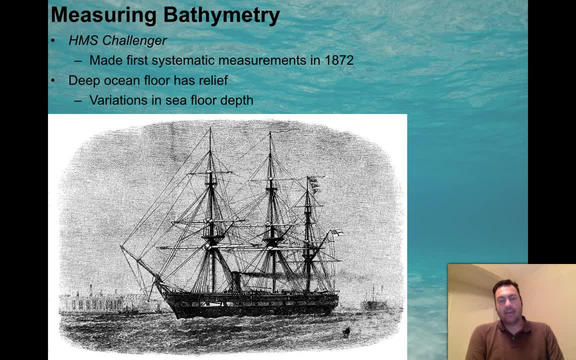 Okay. So some of the most systematic and most important early measurements were taken by a ship by the name of the HMS Challenger. This was done in 1872.. This is a woodcut drawing of the HMS Challenger. It's kind of a really neat research vessel. Not only did it have the ability, 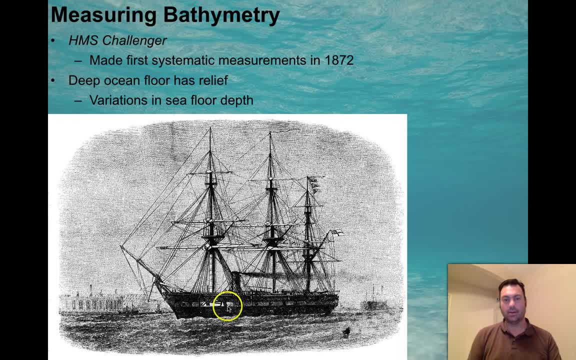 to act as a warship. you can see that little cannon portholes right here- but it had rigging for being propelled by air, by wind, currents, but it also had a steam engine, So it had the ability to be powered. 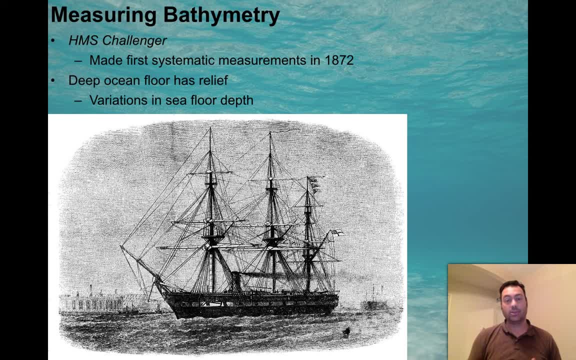 Whether there was any wind or not, And so it was a preferable platform for doing oceanographic research. And what they discovered when they went out is that the deep ocean floor has relief, In other words, variations in seafloor depth. It would go from really, really low, maybe into a. 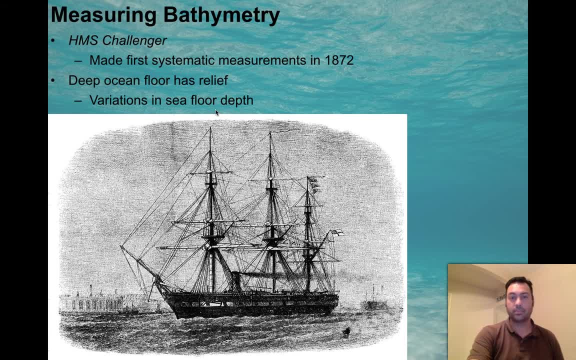 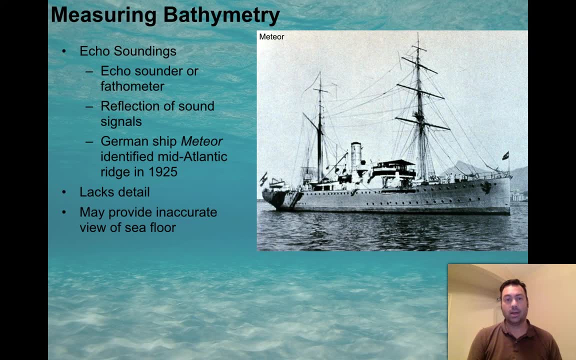 basin and possibly up over a hill. We would get some new technology in the 20th century. One of the first things that we did was we would get some new technology in the 20th century. One of the first things that we did was we would get some new technology in the 20th century. 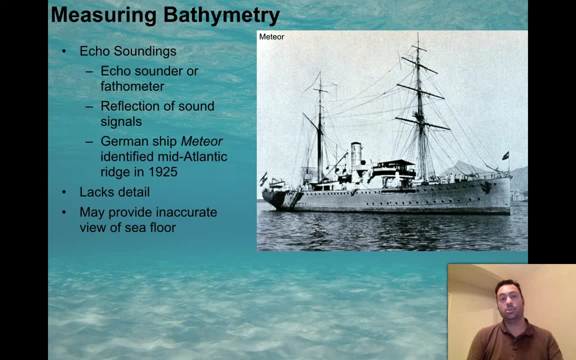 One of the better ships that were used at this time was an old German gunboat from World War I. It was converted to a research vessel. It was never used in World War I, It wasn't finished. Called the Meteor And on this old, this boat that's been used for research, they put in a thing called. 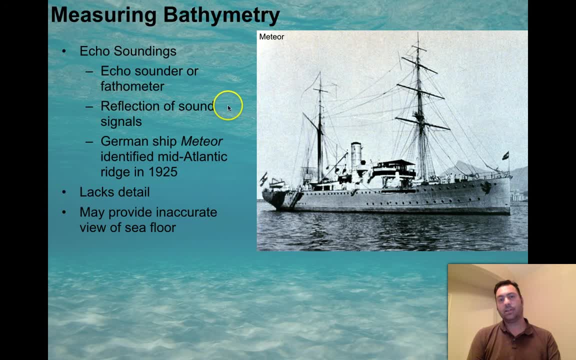 an echo sounder or a fathometer And basically it would bounce a sound off of the bottom of the boat or it would emit it from the bottom of the boat. It would bounce off the seafloor and reflect back up. 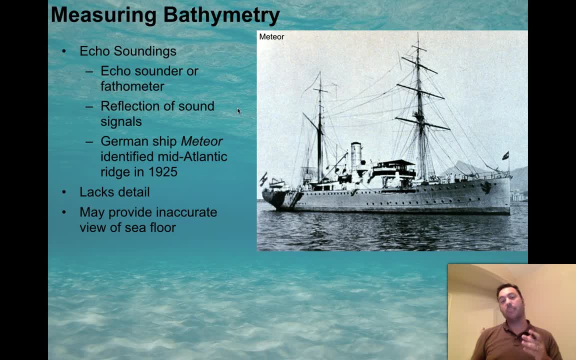 And it would take measurements of the amount of time it would take for it to go down and then come back up. And if you knew about how fast the speed of sound was in water, you could figure out how deep the water was. The problem is is that it lacks a lot of detail and it may provide an inaccurate view of the seafloor. 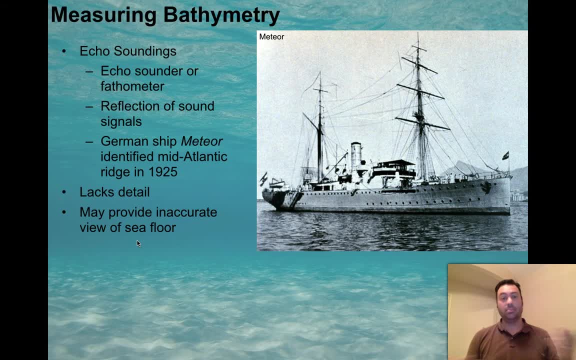 It might give us an idea that something's going on that we don't. that is not completely true. So, anyways, this is the Meteor, and one of the cool things that it did identify was the existence of something called the Mid-Atlantic Ridge. 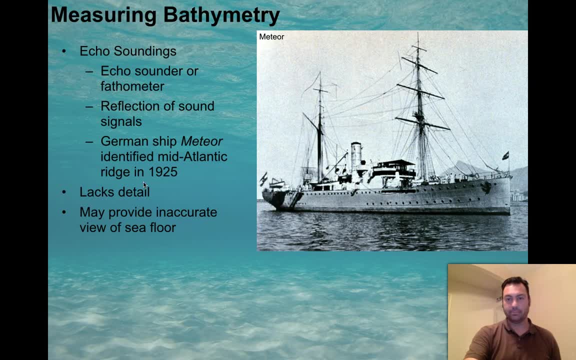 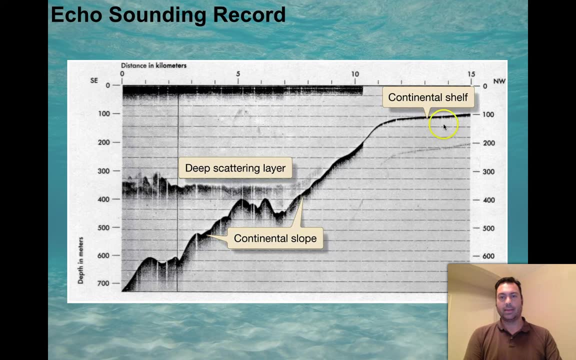 In other words a large mountain chain in the middle of the Atlantic Ocean. So this would be an echo sounding record. That would have been pretty typical at that time. So here we see, the water would be up here at the top. This is, you know, where the boat would be and it would be doing echo sounding. 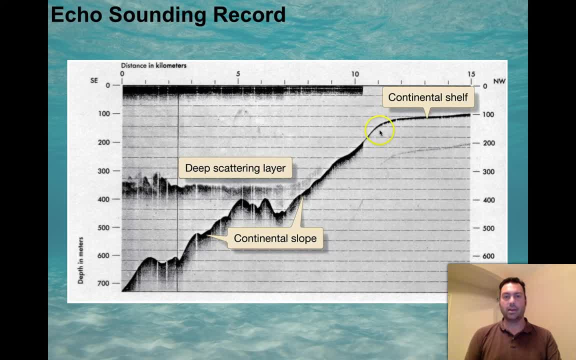 And the continental shelf. we'll be talking about the continental shelf very, very soon. actually We don't want to jump into that just yet, but just right at the edge of the continent we can see that that's underwater. This is land, water, land, water, land, water. 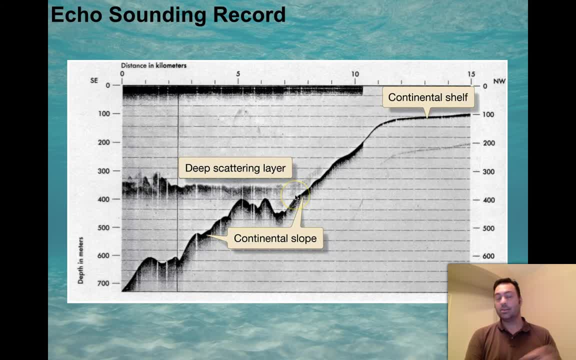 But all of a sudden we see this thing called the deep scattering layer, Something that wasn't actually fully understood until the 1960s and 1970s, But if you weren't careful, you'd think that this was the land surface. 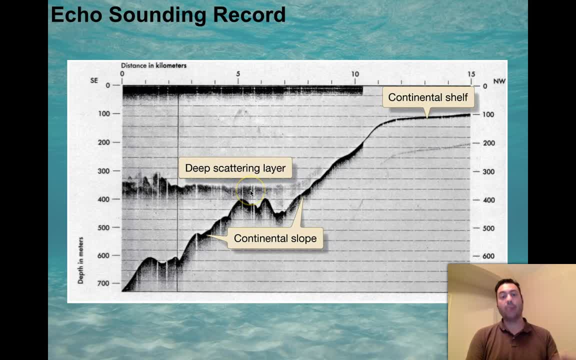 Well, it turns out that this is a phenomenon that has to do with the water and actually the life that lives within the water. The true surface of the land continued down right here. So Echo sounding had its positives, and it also had things that were a little confusing about it. 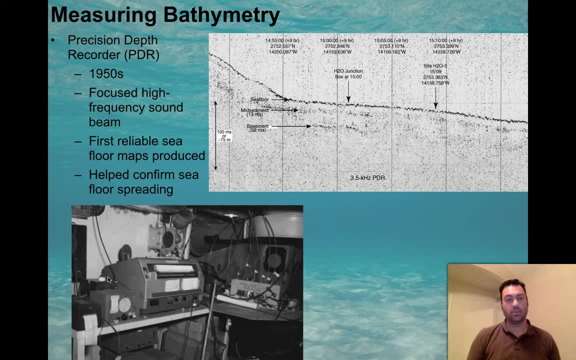 We've developed new technologies, the precision depth recorder, for example, which would be something that you could turn on and run while you were running across the oceans. This was developed in the 1950s and in this case, it focused high-frequency sound beam in a direct location, right. 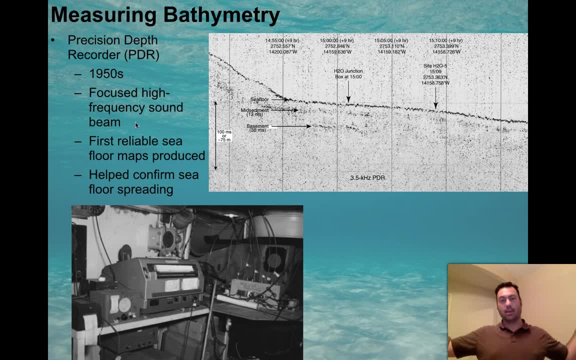 So we can do a transect directly under the boat rather than just making a big splashy sound that went all over the ocean. So it was pretty directed And it gave us some pretty good results. It was the first reliable seafloor maps produced from this data. 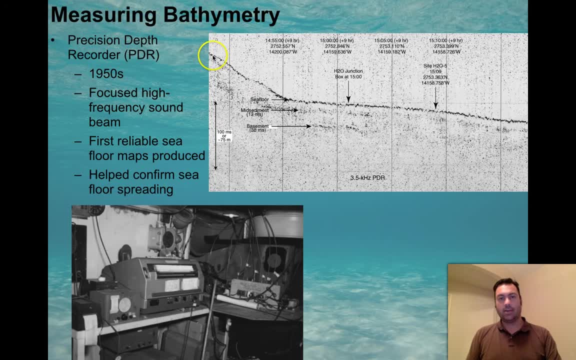 And here we actually learned that we can figure out that not only did we see the water to the seafloor, so here's the seafloor, but it turns out that you can also see that there's layers. Some of these sound waves could actually penetrate into the geology. 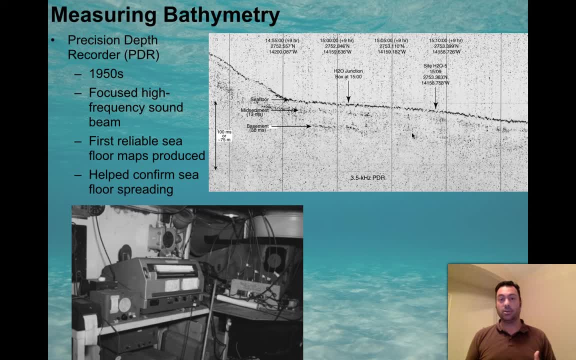 and give us some idea of the architecture of the bottoms of the ocean, So that it wasn't just flat. we can actually see seafloor Here. we would see, you know, a sedimentary layer sitting on top and then finally down below would be the basement. 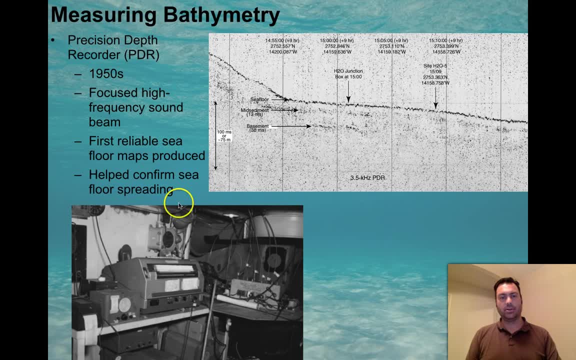 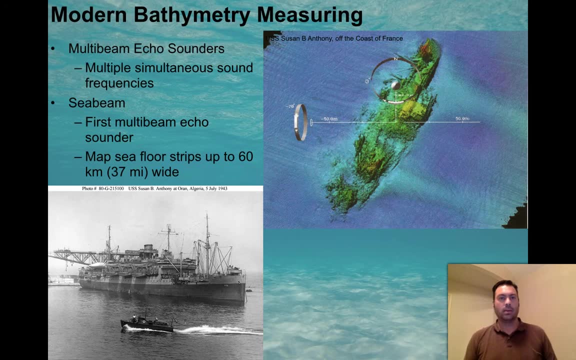 And this was also used to help confirm seafloor spreading. So here's a PDR loaded on a ship in the 1950s. Today we use some newer technology, that kind of supplants both of those. We still use those to a certain extent. 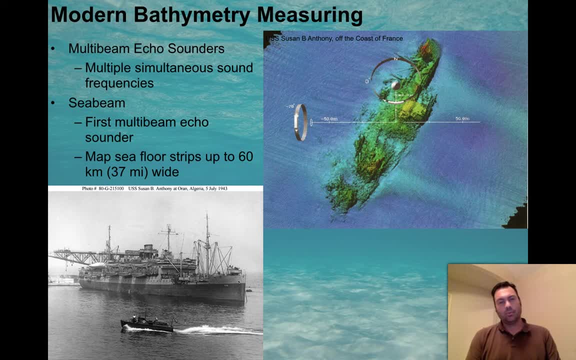 especially in more simplistic analysis. But real oceanographic research uses some really neat technology: Multi-beam echo sounders, which are multiple simultaneous sound frequencies. So in other words, instead of using a single frequency, we use a number of frequencies and bounce them off the seafloor. 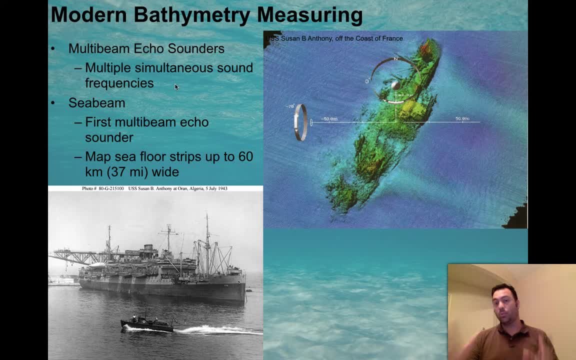 And that allows us to see more than just weight, for example, where the wood is or where the metal is in the case of a shipwreck. So here we see a shipwreck, The USS Susan B Anthony, which is off the coast of France. 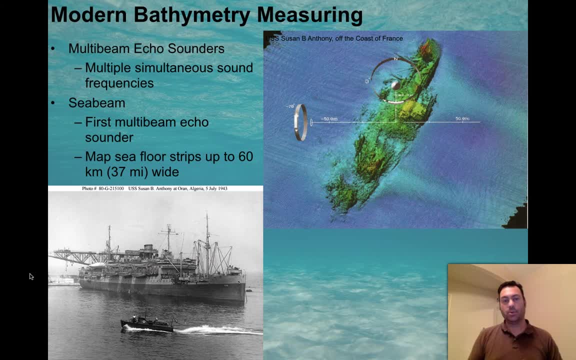 This is the Susan B Anthony over here. It was a ship that was destroyed during World War II And you can see that by using multi-beam, or in this case C-beam, the multi-beam echo sounder, we can see some details in here, different materials that would have been exhibited on the original boat. 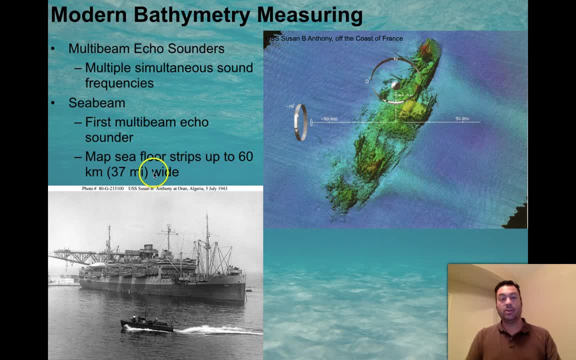 So it allowed us to map the seafloor up to in stripes, up to 60 kilometers wide. The seafloor is very, very wide, So this was a really great technique and it gave us some really nice detail that we could use to look at the seafloor. 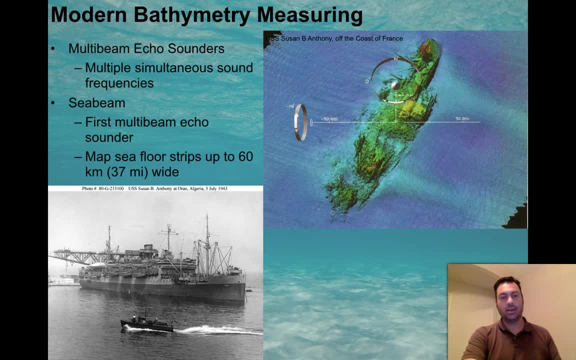 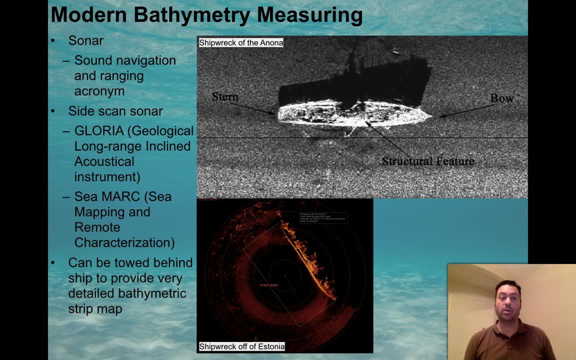 This is a fairly large ship, but we'll find that the technology as it exists today is even better than this. We started developing real sonar as we know it today, which is a sound navigation and ranging acronym right Sonar, And so the main ones that we use for exploring the seafloor in. 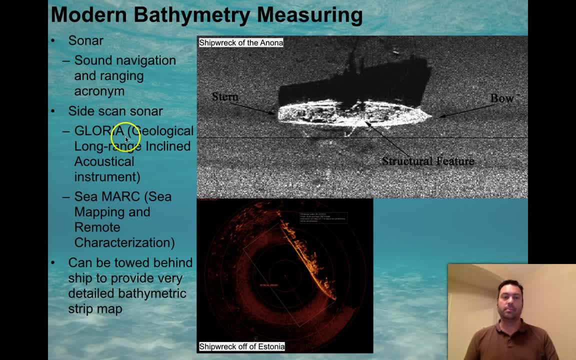 Oceanographic research is side-scan sonar Gloria, which is an important one to know, SeaMark. Basically, these are able to get extremely high-resolution images. Here we see a shipwreck of a very- it's about 150 foot, if I can remember, about 150 foot- yacht that had sunk into the ocean. 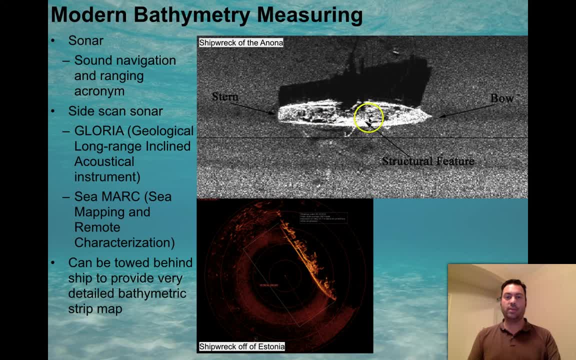 And here we can see pretty good detail of the yacht From the surface, From the surface of the ocean. Here's the back of it, Here's the front of it. We see some structural features And actually things on the deck as well, scattered around. 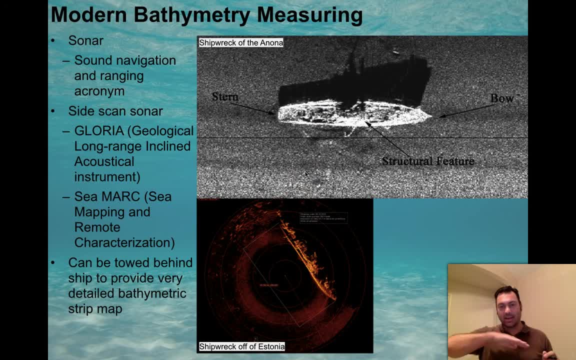 And remember, because it's a side scanner, it comes in from the side, So it actually produces a shadow over here, a sound shadow in the sonar that we can see The other here we can see another one. This is a shipwreck off of the coast of Estonia, which is near Russia. 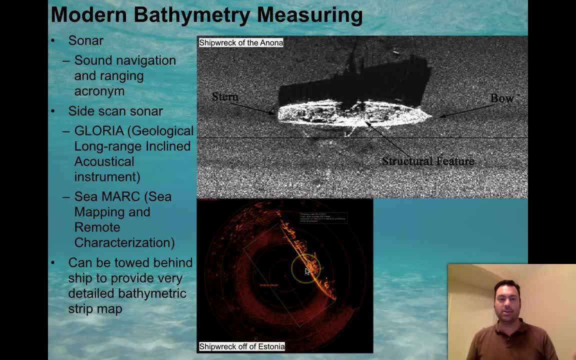 Again, we can see very good detail And these can be towed behind the ship to provide very detailed bathymetric strip maps. So as the ship is going across the ocean, this thing can be dragged behind far away from where the propellers are going to produce a lot of static. 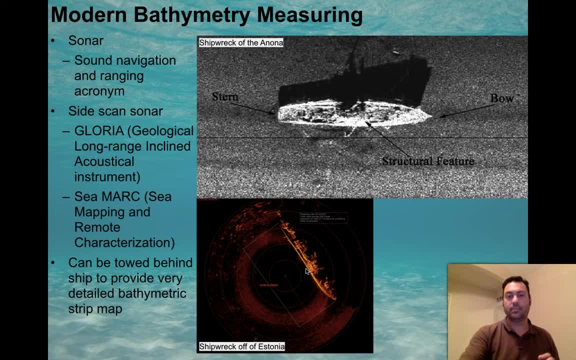 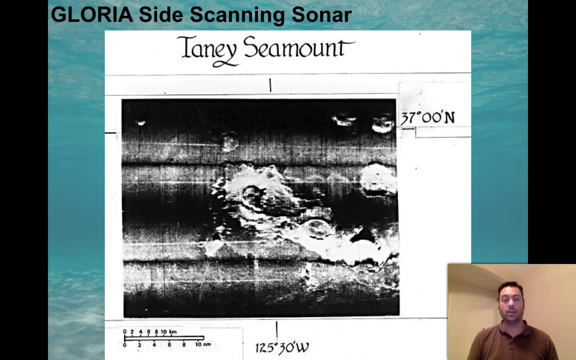 And you can get some really good images. Here's an early image of a seamount. This would be an underground or, I'm sorry, underwater volcano- Something sitting on the seafloor. Here we can see the crater up on top. 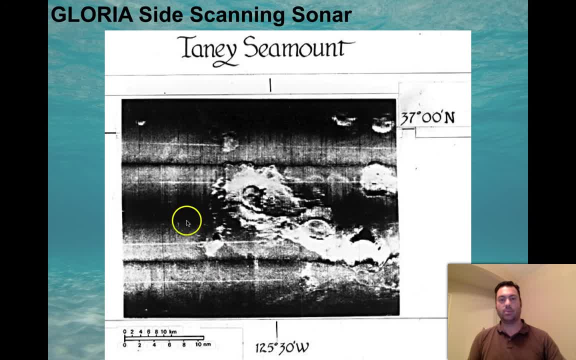 And here we see this big, wide swath. This is actually a nice big, wide swath And we get a really good sonar image- using Gloria in this case- of the seamount. We can even see the size of it, right. 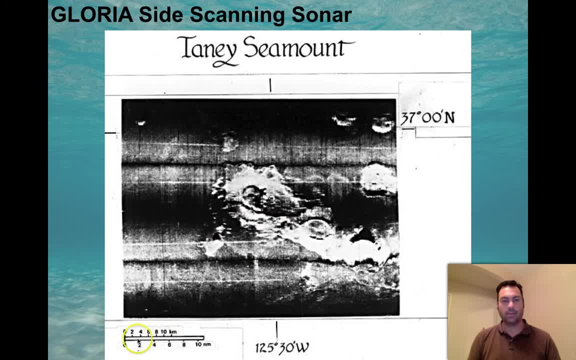 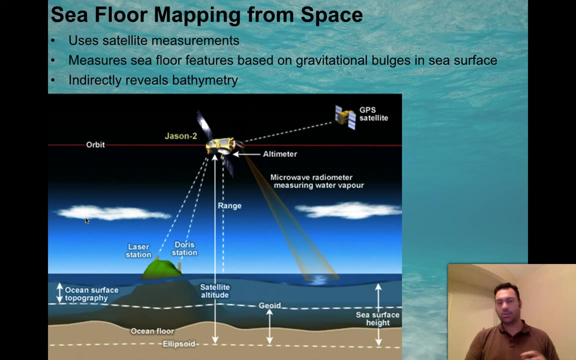 So this is a fairly large feature, about 10 miles across. So this is about 10 miles. also, right here, Very large seamount which is basically a volcano on the seafloor. So that's one way of mapping things. It's just simply. 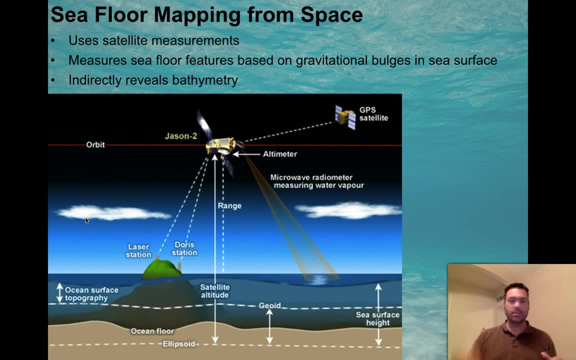 Take a boat around and take all kinds of sonar measurements, do depth soundings and put all that stuff together and get a good map. But there's also another way we can do it that's even more efficient, And that is we can use satellites. 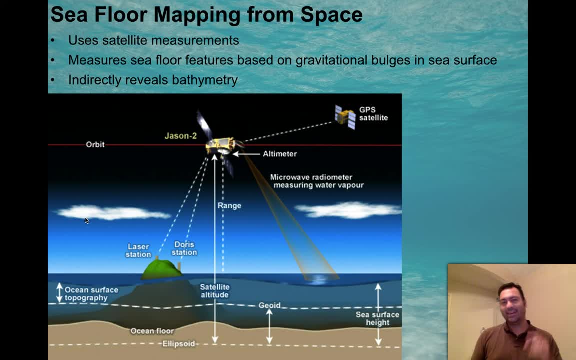 You might be asking yourself, the satellites can actually see to the bottom of the ocean- Not directly. It turns out that the Earth's gravity field is not exactly the same everywhere on the planet. If you happen to be in an area Where there's large mountains, the gravity of the mountains is added to the gravity of the Earth and it's slightly stronger in those areas. 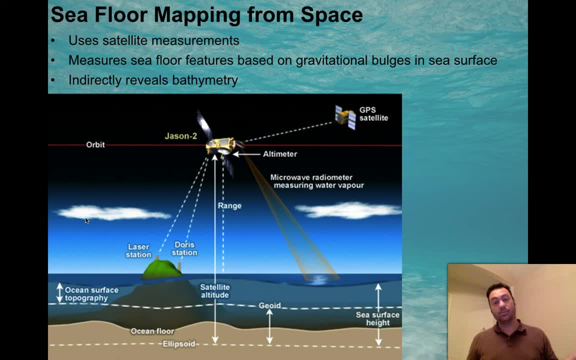 In other places, where there's a big basin, the gravity is slightly reduced. So what does that mean? Well, that means that if the bottom of the ocean has the same features- mountains and basins and things like this- It means that there's going to be a varying gravity field across the surface of the ocean, which means that the ocean, in some places, will be pulled down preferentially by the Earth. 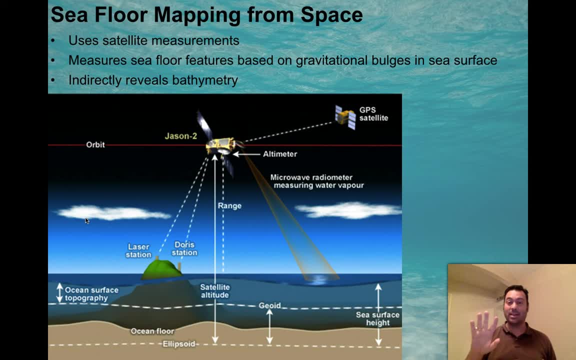 A little bit more in one area than it will be in another. The amount of that is very, very small. You know the amount of sea level change will be very, very small, But it is, it turns out, measurable All the way from space. 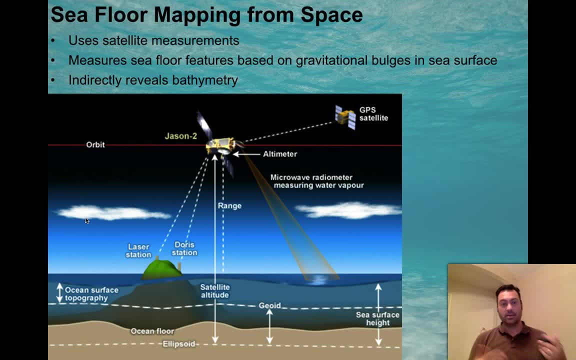 As a matter of fact, we get the best measurements from space in doing this. The satellite that is most famous for this is the Jason 2 satellite, which has been in orbit for a while, And we've got a wonderful seafloor map. 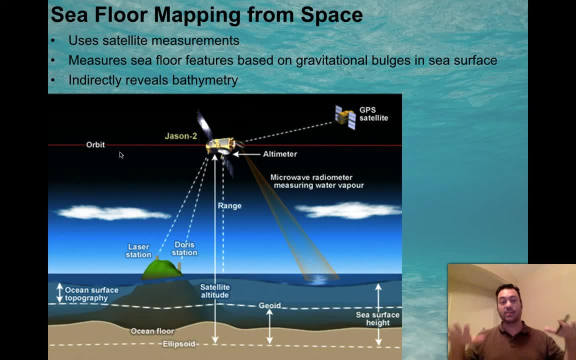 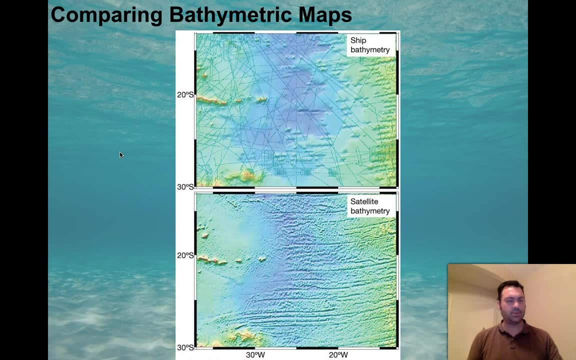 From looking at the gravity, The gravitational effect And all the effects of the surface of the ocean. And so what do we see? Well, this is the difference, right. So here we see the ships, The ships going around dropping sonar, you know, taking sonar measurements, doing depth soundings, and actually these lines here are where the research vessels have been right. 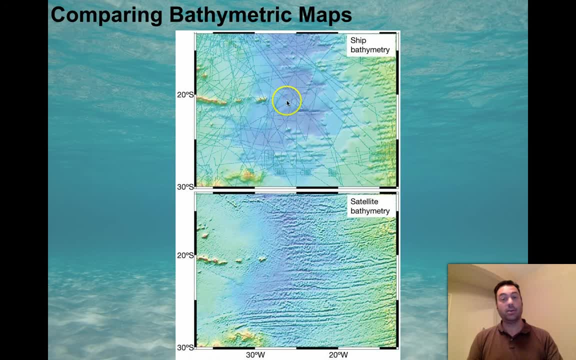 You'd actually have to take a ship literally up and down everywhere to get a perfect map. It's very difficult and very expensive. A satellite, however, goes over it. Every you know it might orbit the Earth every 90 minutes. 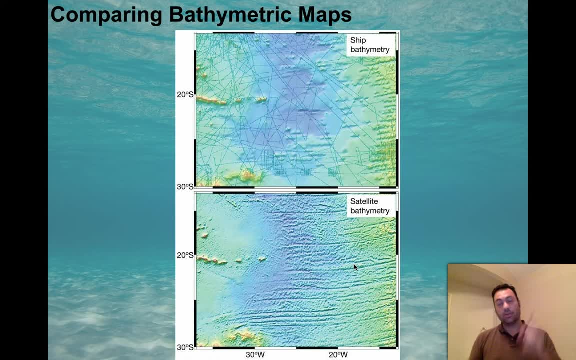 If it's a geostationary satellite, it means that it sits over the Earth in the same place and it gets a very good measurement. It's constantly monitoring And we wind up. this is the same image or, I'm sorry, the same location, but measured by two different things. 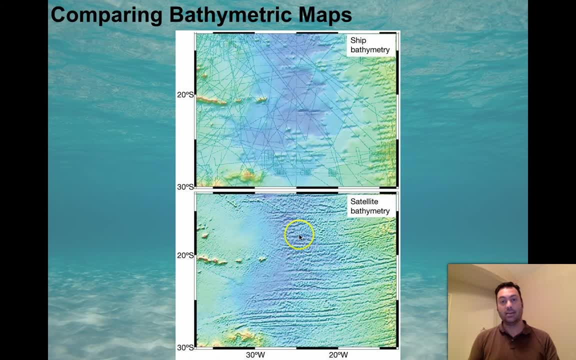 We can see that the satellite actually picks up tremendous detail, Much of which is lost by the ship bathymetry. So right now, the preferred method is, to strange as it is, to indirectly look at the curvature of the surface of the ocean based upon the gravity, rather than to just simply go out and drop the sounding device into the water. 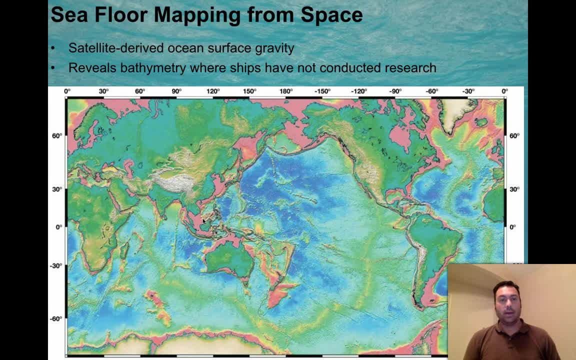 All right. So we've got some really cool stuff from this. You know we've got a wonderful understanding now of the sea floor. These blue areas here are obvious. Well, let's give a little kind of coding of what's happening here. 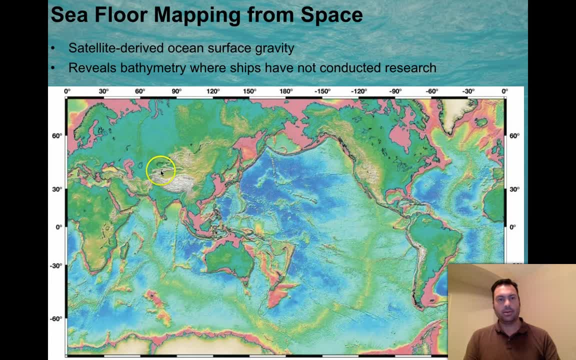 Let's see if I can get my There. it is This: here is Asia, Africa, North America, South America and Australia. This is the Pacific Ocean right here. The Pacific Ocean actually comes down over here And we'll notice that the Pacific Ocean right down here has a nice high grounding area. 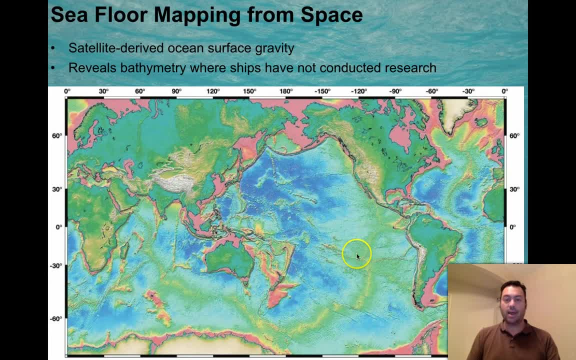 And over here in the blue it's nice and low. This high ground that's located over here in the southeast is the East Pacific Rise. It's a mountain range. It's a very wide and tall mountain range, but it's still a mountain range. 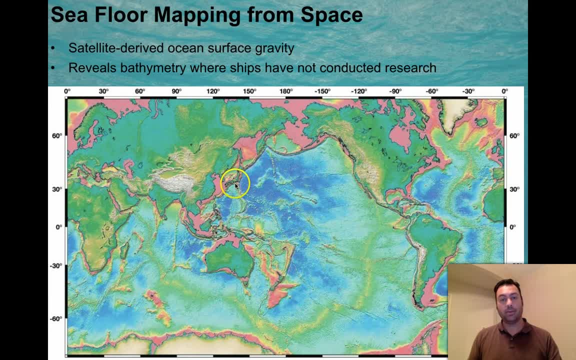 Whereas when we come over here, near Japan, Japan- Japan being located right here- We find that this blue area is actually a really deep basin. It's actually quite deep, And the deepest place on Earth is located right here, next to these islands called the Marianas Trench. 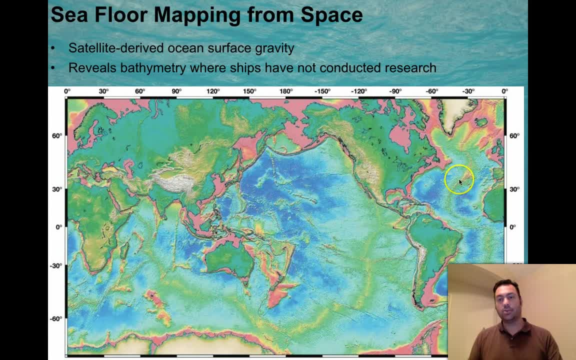 Here we see the same features. Right here, this is the Atlantic Ocean And right in the middle is the Mid-Atlantic Ridge, Coming right through the middle here. we see a blue basin over here, meaning that it's deep. It's deep here. 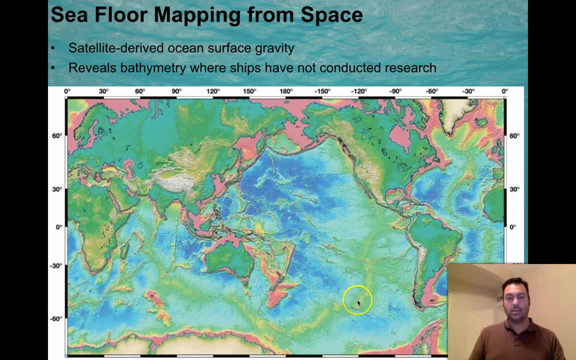 This is where we begin here. Okay, So this is where the sea floor spreading is occurring on planet Earth, At the tops of these ridges, Alright, And they're spreading in this direction, and this direction in the case of the Pacific. 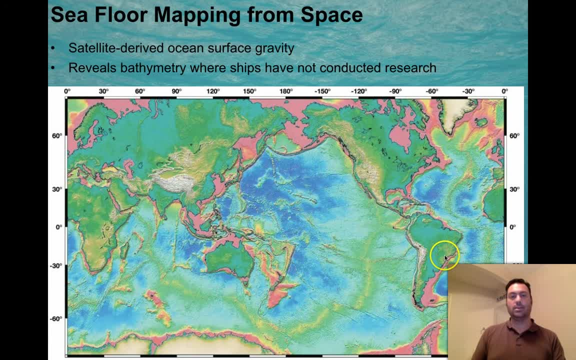 And from to the west and to the east. in the case of the Atlantic, It gets a little more sophisticated when we get into the Indian Ocean, Alright, But the beauty of this is that we have got amazing bathymetry. We have a really good understanding of what the bottom of the oceans look like. 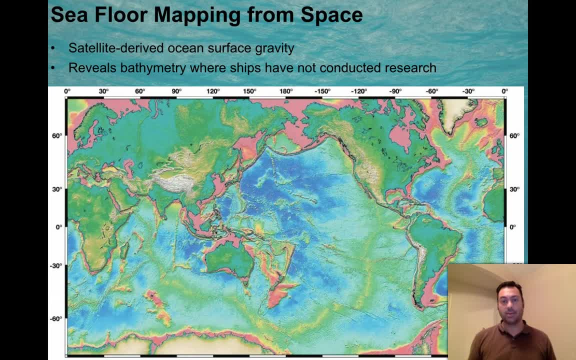 And we go out and test it by seeing if, in fact, the seamounts are there. We do in fact, find that the satellites have found things that we could otherwise find. It's awesome, It's a really awesome technology. 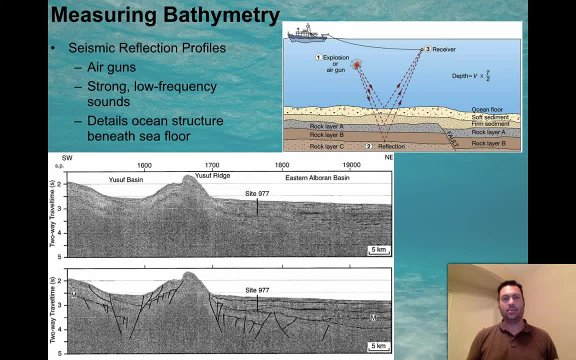 So how does it work? What is the general idea of measuring bathymetry? Well, there's a couple of ways you can do it. The most common way that we do it to be able to figure out what's going on, Say, in the earth. 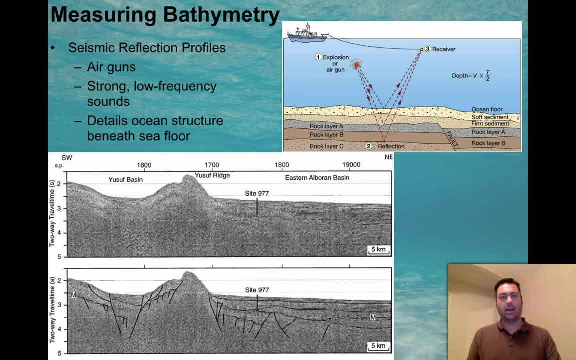 Down deep below the water Is we use something called an air gun Right. An air gun is something that puts a blast of air into the water column. There's my stylus. An air gun puts a blast of air into or an explosion. you can use dynamite too. 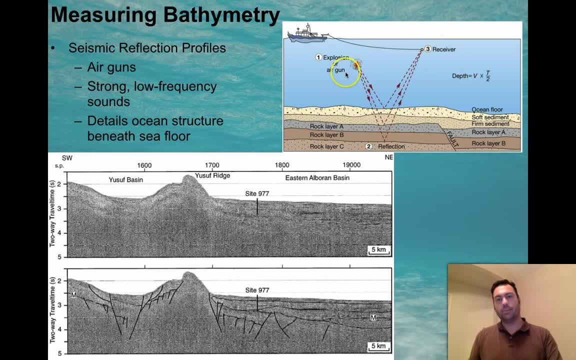 It puts a shock wave through the water And that shock wave is able to penetrate through the water and into the rocks and off the layers And reflect back to a receiver And the receiver simply looks at the different frequencies that come in And the times at which they come in. 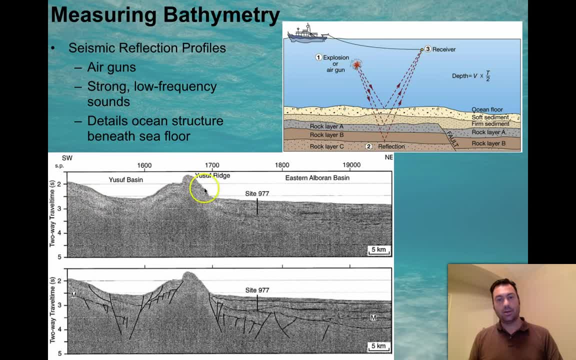 And we can get some really cool stuff. So this is a picture of a basin And I believe this is a basin in Alaska, If I can remember. I might be wrong about this, But anyways, But there's a basin And we're able to actually come in and figure out where the faults are. 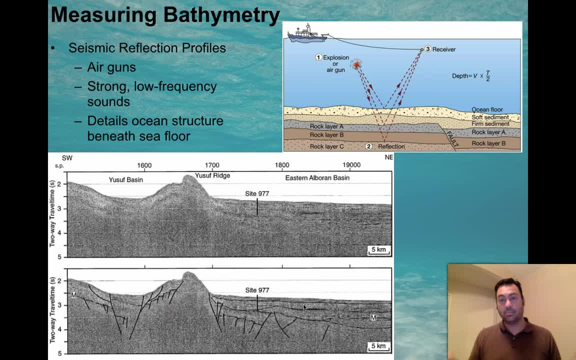 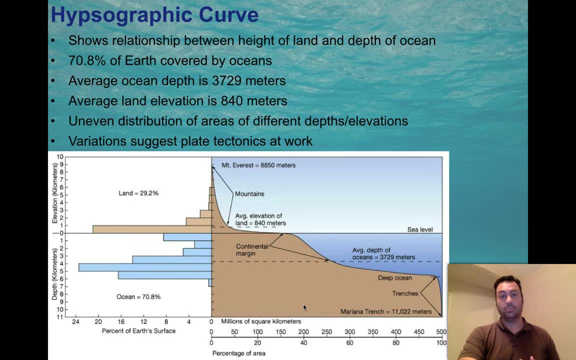 And how things are broken up And put an interpretation of what's happening here. So not only do we can see the depth, We can actually go into the rocks below. Really cool, Alright. So now that we've kind of got an understanding of how we know what the bottom of the oceans look like, 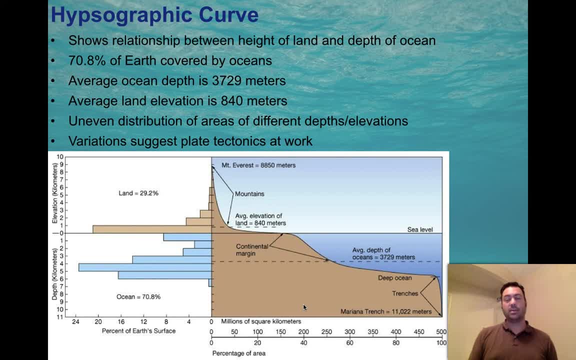 Let's talk about what we've discovered from that, And some of the things are kind of interesting. Let's talk about the hypsographic curve first off. It shows the relationship between the height of land and the depth of ocean. So 70.8, or about 71%, of Earth is covered by oceans. 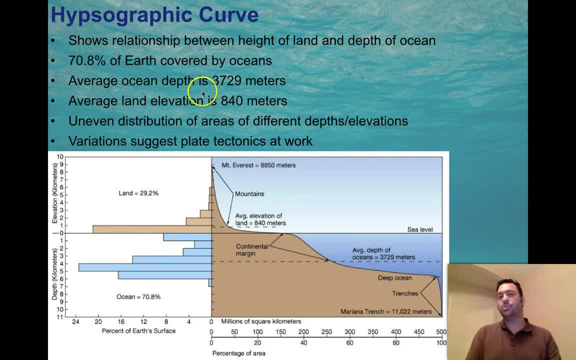 So we've learned that We also learned. the average ocean depth is 3,729 meters. That stands in contrast with the average land elevation, Which is 840 meters. It means that the Earth is almost covered with water. Right 71% of it is already covered with water. 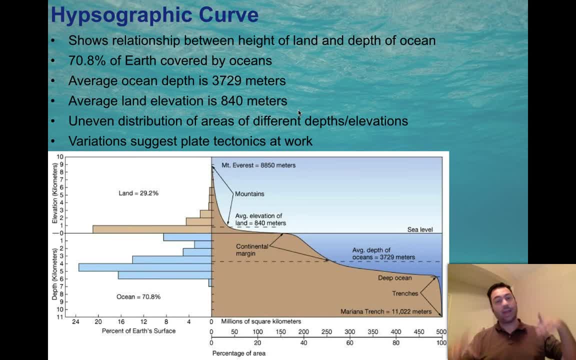 The land is really just sticking out, The continents really just happen to be sticking out of the surface of the oceans. Okay, Uneven distribution of areas of different depths, Depths and elevations. In other words, not everything on the bottom of the ocean is nice and flat. 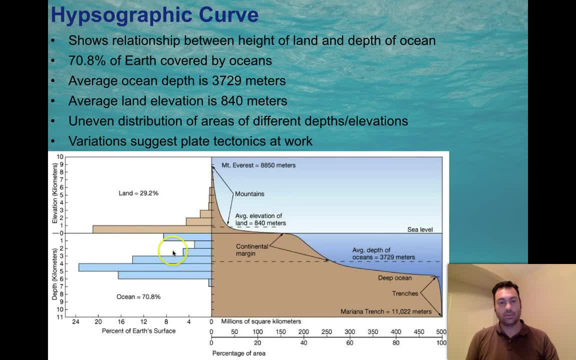 It turns out that when we look at the hypsographic curve- Which is right here for oceans, Those depths at any given location on Earth has a wide variety of landscapes, A wide variety of depths, And there's no uniformity there, Right. 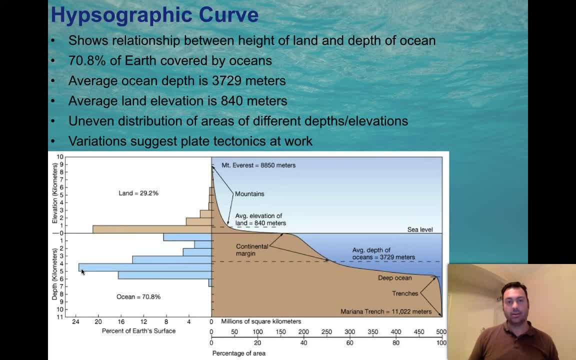 It's not like you go into the ocean and it goes right down to five miles and stays there. There's all kinds of stuff happening, And the variations suggest plate tectonics at work. Cool, Alright. What have we learned from that then? 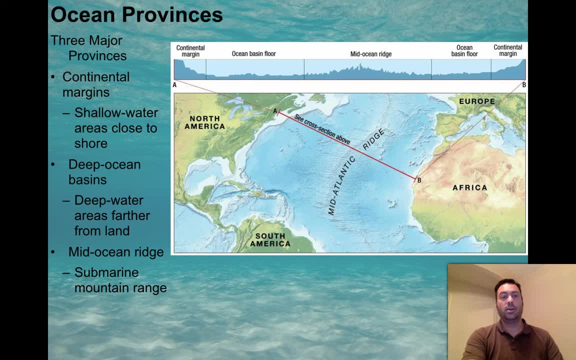 What have we learned from all of this stuff, All of our research and our work? We've learned that there's three major provinces in the oceans. So when we look at a cross section of, say, the Atlantic, So here we have the Mid-Atlantic Ridge. 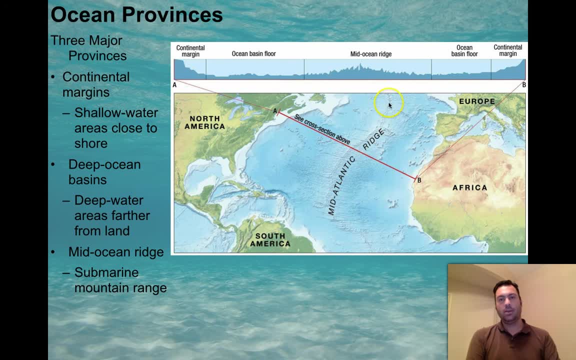 Located right in the middle of the Atlantic Ocean. We discover that this is the cross section right here. That here's the Mid-Atlantic Ridge. It's nice and high, It's the longest mountain chain on the entire planet And it's right in the middle. 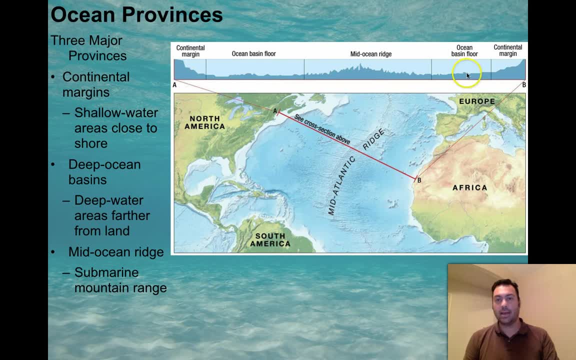 But as we go to the west and as we go to the east It sinks down and we have a nice basin on both sides. So here and then, as we hit that basin, We head up into the continent in something called the continental margin. 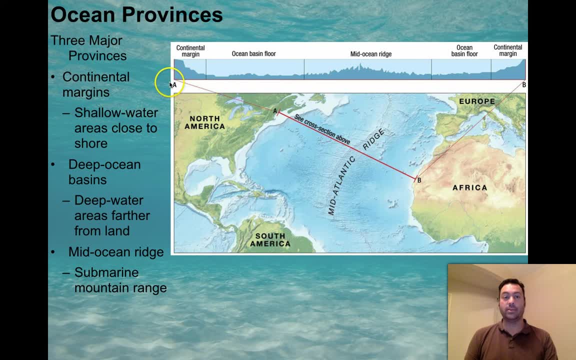 So we divide the oceans generally into three provinces: The margins right next to where the continents are, Which is also where a lot of the life is And where a lot of the important economic activity occurs. The ocean basin floor, Which are these wide areas that tend to be relatively flat. 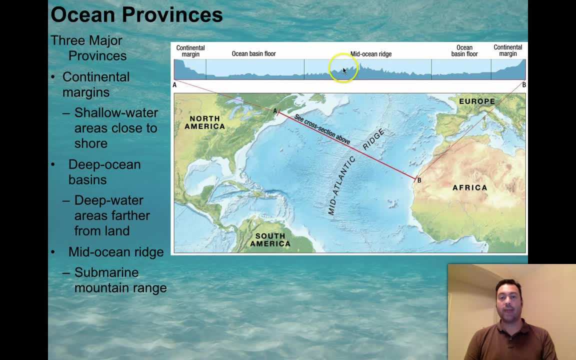 And usually in the middle, right where the ridge is. If there happens to be a ridge in that ocean, You get it right here in the middle And it tends to be quite tall, And then you get another ocean basin floor on the other side. 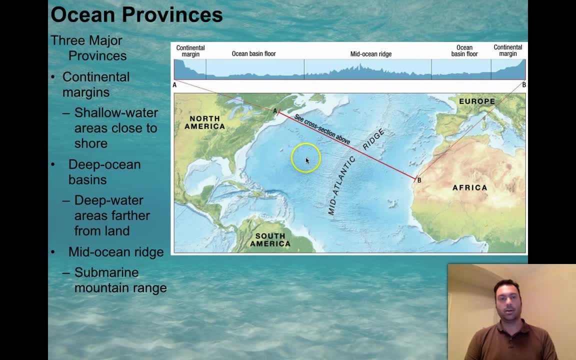 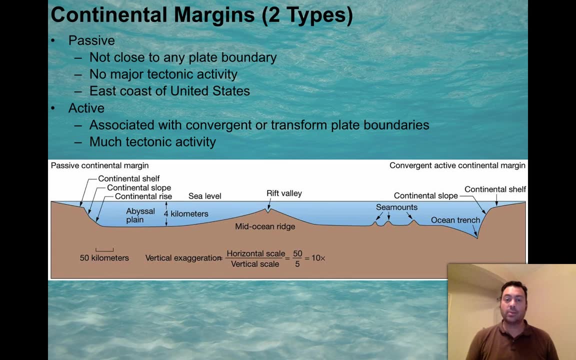 And another continental margin, As we see from Africa to North America. Okay, So one of the things we're going to do Is we're going to actually go through systematically each type. The first type we're going to talk about are the continental margins. 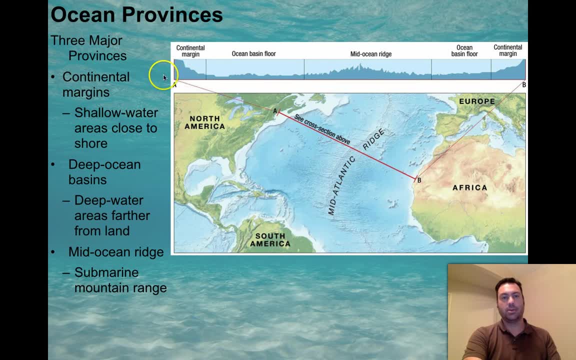 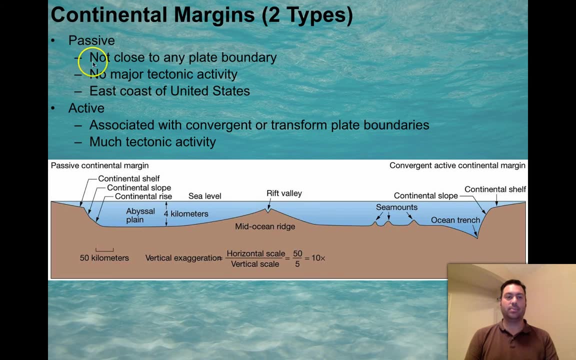 So, remember, we've got three major provinces. We're going to talk about the margins- This area over here And this area over here- And it turns out there's two different kinds. There's a passive margin that can form, And that's when there's no plate boundary anywhere in the area. 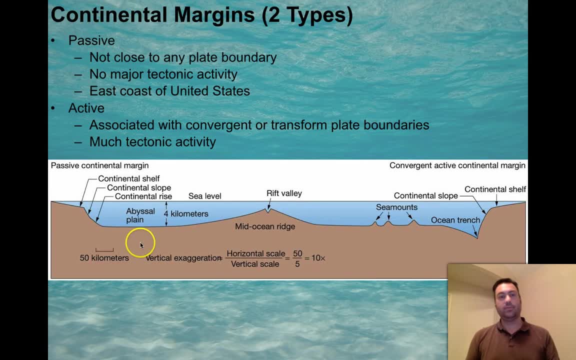 It just happens to be that there's a continent here And here's the sea floor And there's no major tectonic activity present. So east coast of the United States is a classic place that people point to Is where we have passive margins. 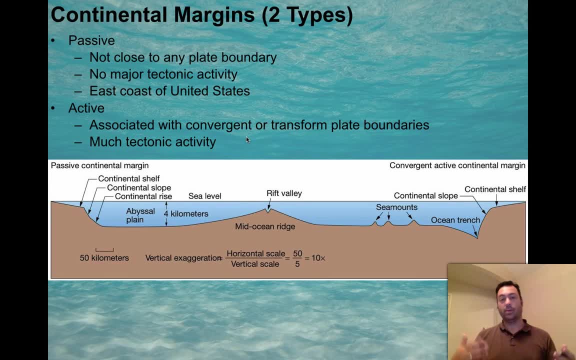 But an active margin is where we have convergence or transform boundaries. In this case, California or Indonesia would be perfect locations to think of convergent. In the case of Indonesia, transform would be the San Andreas Fault of California. There's a lot of tectonic activity in these locations. 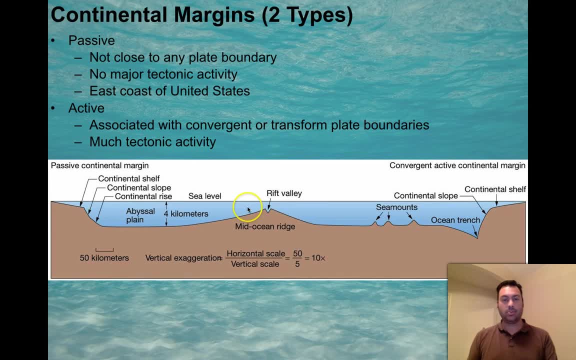 Famous for tectonic activity. So let's see how these would compare. Well, here we have our spreading ridge, Our mid-ocean ridge, Our Rift Valley. Everything over here comes over and just passively connects into a continental shelf, And there's not really a whole lot going on over here. 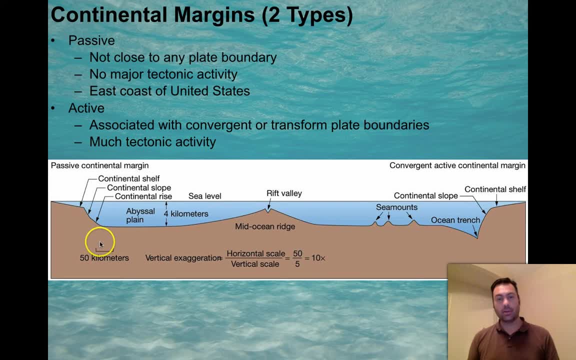 This is not an area where you're going to see a lot of earthquakes or volcanoes. On the other side of this, however, there's going to be sea floor spreading towards another continent, But in this case, the continent is subducting the. 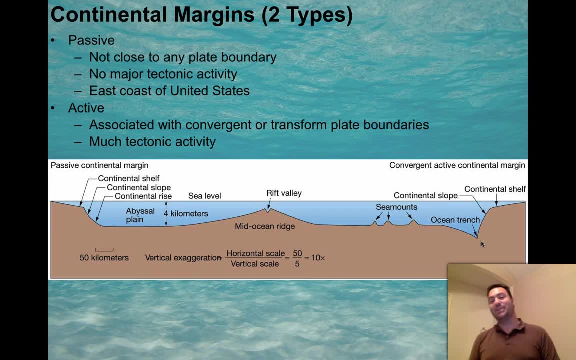 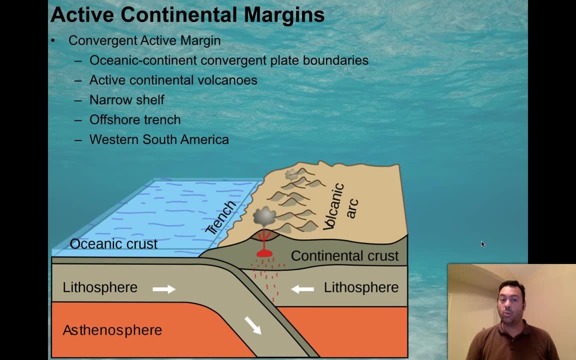 Pacific or not. the Pacific, the oceanic plate beneath the continent, And so you get a lot of activity along the trench. So what is kind of interesting to look at right away is going to be active continental margins. They're extremely important because that's where the tectonism occurs. 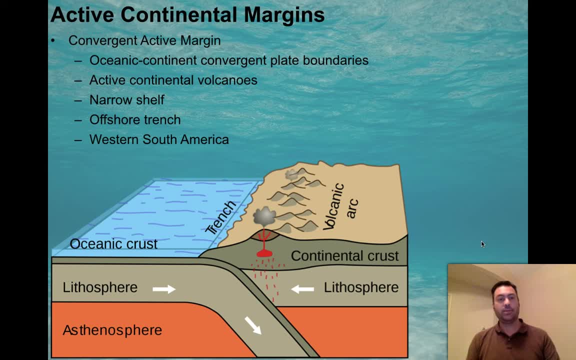 That's where a lot of movement occurs on the Earth's surface And there's different kinds. You can have a margin where you have the oceanic to continental convergent plate boundaries over here. That's what we've got drawn down here. Here we have an oceanic plate that's hitting into the continental crust. 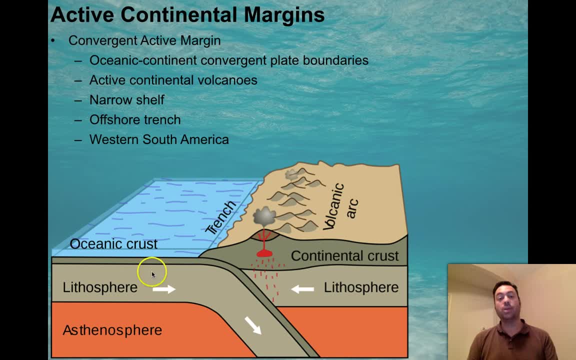 And the lithosphere of the continental plate. I'm sorry, the oceanic plate subducts beneath that of the continental plate. It tends to have a lot of active continental volcanoes right. A lot of volcanoes will form here along this volcanic arc. 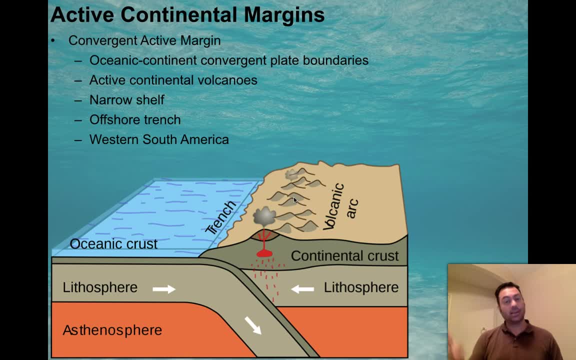 And you'll have a lot of really dangerous Mount St Helens-style-type eruptions happening. A consequence for this is that you get a narrow shelf. In other words, there's no real place that sticks out here into the ocean, where it's shallow water. 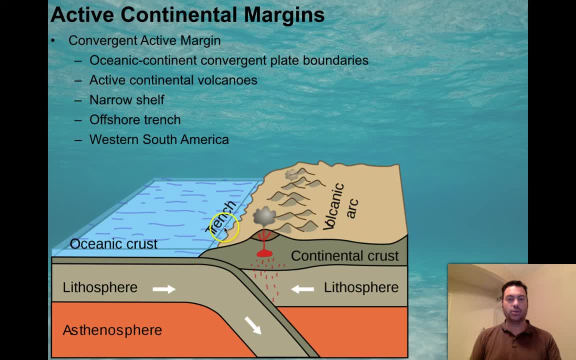 Literally, it falls off from the beach, It goes out of short ways and then it goes right down into the trench And it can be a very deep trench, And that's what we're referring to here- offshore trench- And a classic place where we see this is western South America. 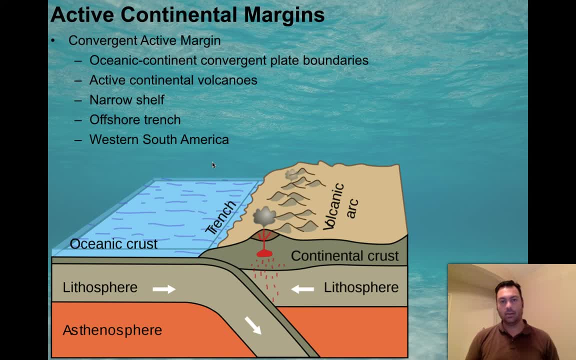 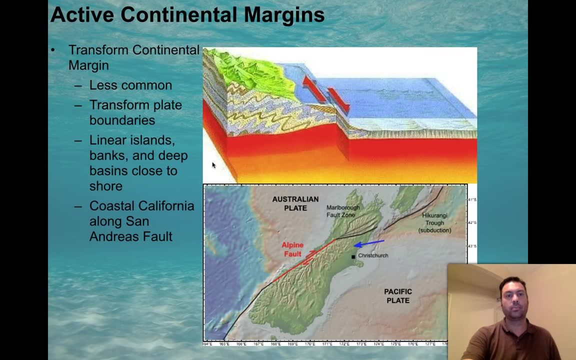 Countries like Chile, and even as far north as Mexico, We see this type of feature. By contrast, we can look at a transformed continental margin right. Sometimes the plates will move past each other rather than one over the other In the case of a subduction zone. 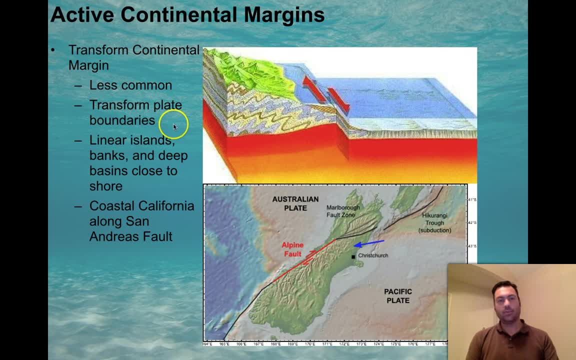 It's less common, but they do happen. The transformed boundaries tend to lead to linear islands, banks and deep basins close to shore. Coastal California along San Andreas Falls is a classic example, But it's not the only place. Down in the South Pacific. there's another great place where we can look at such a relationship. 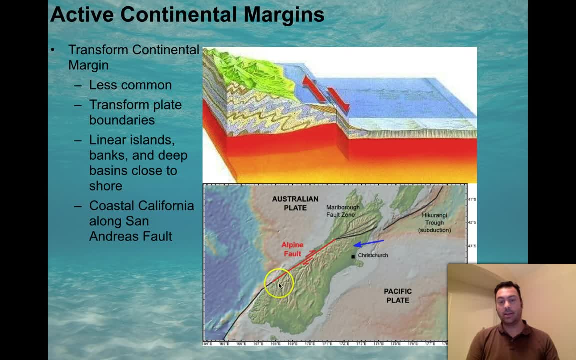 The Alpine Fault which is in New Zealand. New Zealand is largely on the Pacific plate, But on the other side of the island it's on the Australian plate And the two plates are moving past one another. And as it's moving past one another it's popping the land mass up and creating New Zealand. 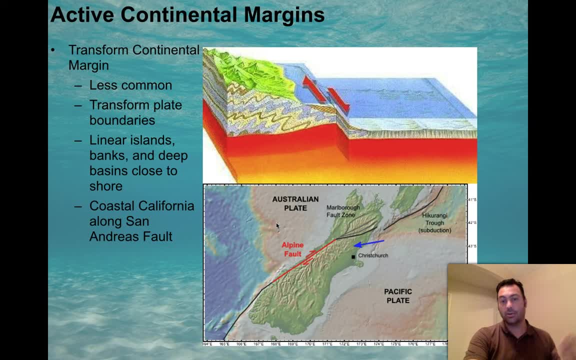 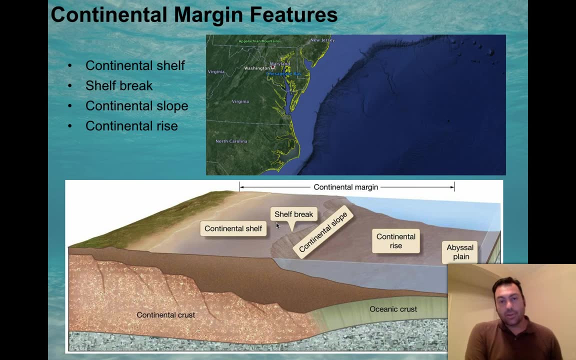 Which is kind of an interesting thing. It's an interesting place to go and visit for geological reasons, right off. So some of the features that we see in a continental margin, in a passive margin, is we will find something called a continental shelf. 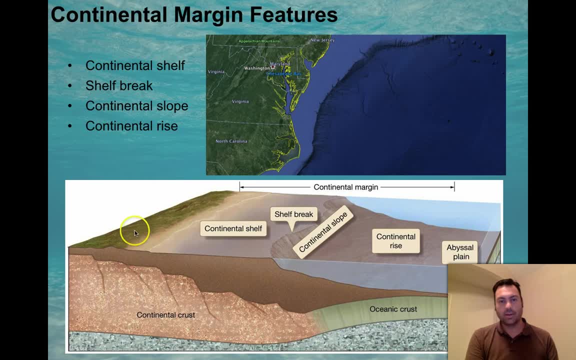 So the continental shelf. here we see the continental crust. The continental shelf is this big pile of sediment that's literally stacked on top of the continental crust And it'll pile up to a certain point And then it'll fall off very abruptly onto the oceanic crust. 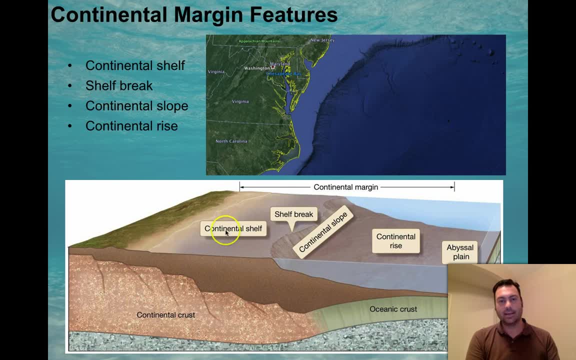 And when we look here at this picture, we can see that the continental shelf extends quite a ways out on this passive margin. Here we see the coast of Virginia and North Carolina And we can see that this continental shelf extends way out to about this point right here. 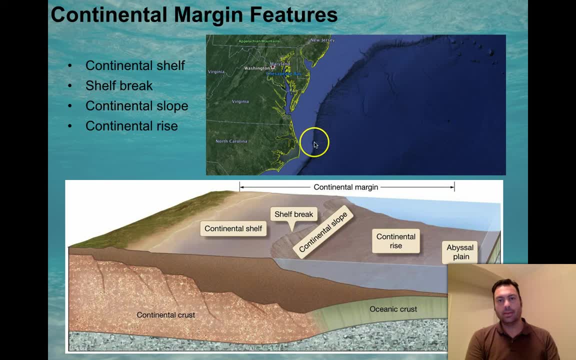 This line on this map up here is the edge of the continental shelf, Until it hits something called the shelf break. This is the shelf break, And so we see that sudden drop off towards the deep water That's located right along here, And then we see the continental slope. is this region right in here? 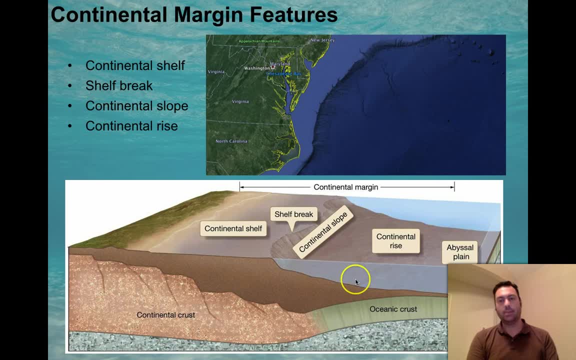 Where the sediment is still actively piling up. You see this piling up area right here, And then, down at the bottom part, we get the continental rise, Which is located out over here. Finally, you get out into the abyssal plain, which is the deep water. 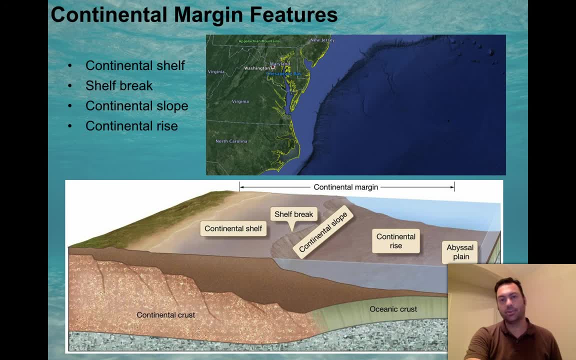 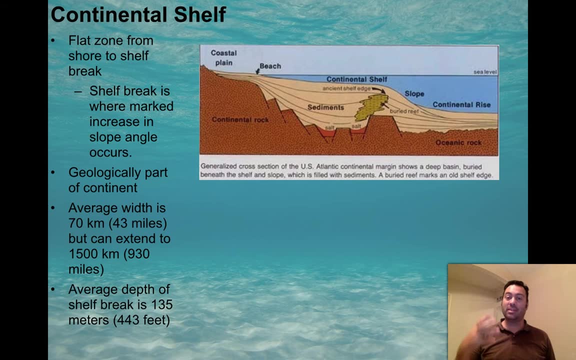 So this is typical passive margin features. So to really have an understanding of these features, we're going to take a quick moment to kind of cover the major aspects of them. Because in politics and law- international law of the sea, or just in development of economic resources, 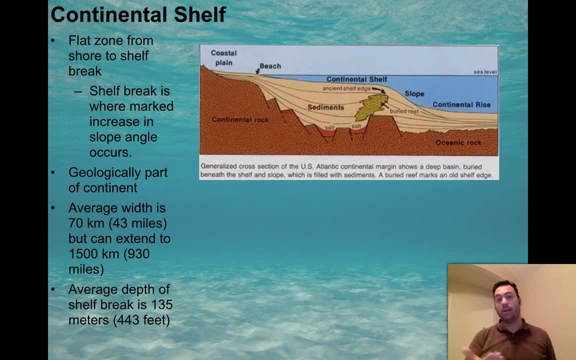 the continental shelf is where a lot of the good stuff that we like to mine in the oceans is located, And it's a place of tremendous friction and controversy between countries, even to this very day. We see it playing out currently in the South China Sea. 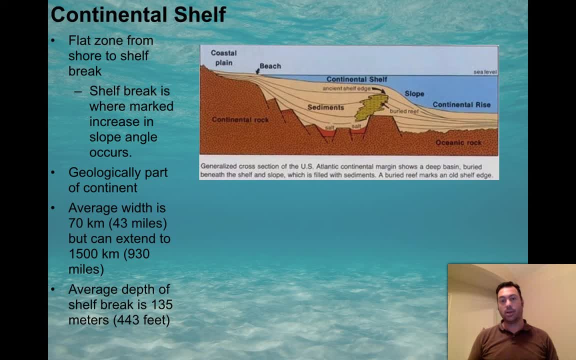 And in territorial arguments between the Chinese, the Japanese, the Filipinos and the Vietnamese. So what is the continental shelf then? You know, I kind of went over it really quickly. Well, it's just simply the flat zone from the shore to the shelf break. 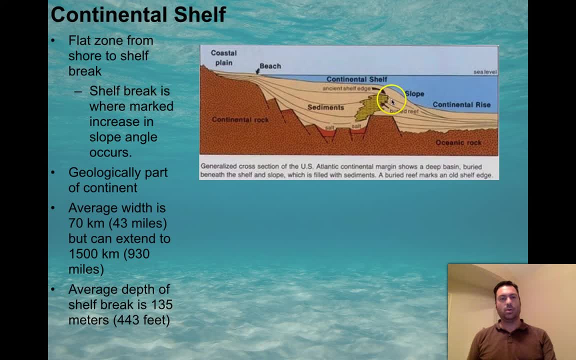 We talked about the shelf break as where it goes off into the deeper water. Geologically it's part of the continent. So if you're, If your country happens to be located here, the argument is this is geologically related to it. 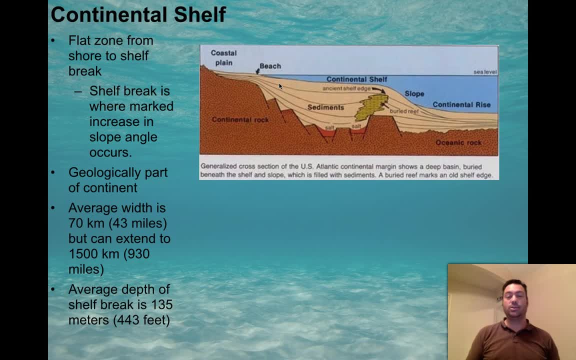 And therefore you can have access to this, But perhaps in certain conditions your neighbors also have access to it, Or in other conditions maybe not. It's kind of a complicated argument. The average width is about 43 miles, But can extend 930 miles out, right? 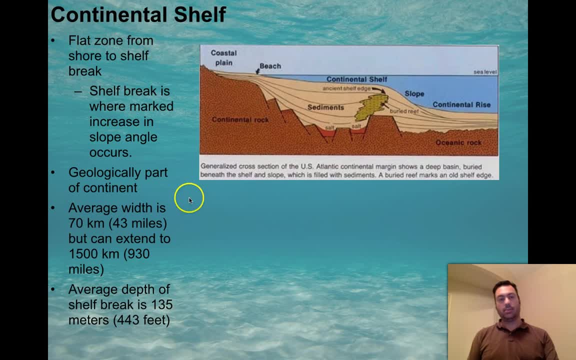 So this is just a very thin wedge of water sitting on top. The average depth of the shelf break is about 400 meters- 443 feet. Once you hit about 443 feet depth, usually it drops right off into the deep ocean. Okay. 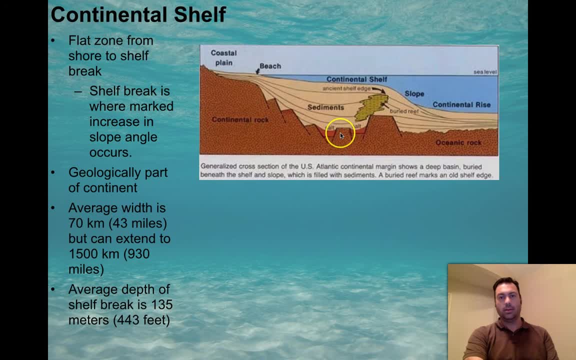 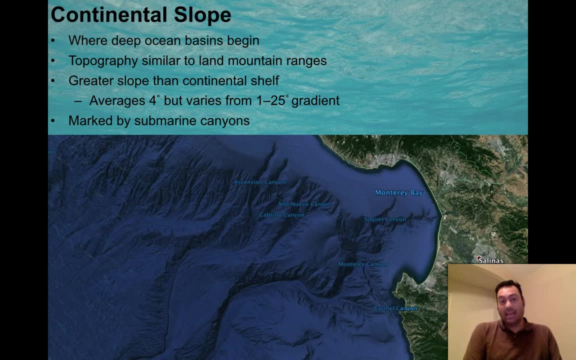 So that region right here is where all the goodies are that we like to mine in the ocean. The continental slope is where the ocean basins begin Right. So here we see the nice shelf. This is off the coast of California- And then we go off into this nice slope. 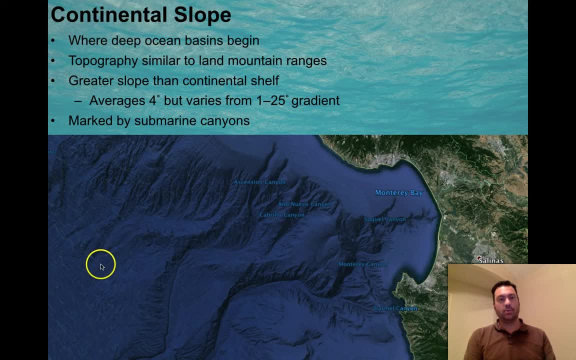 Right, And this is the stuff that's dropping down to the sea floor. The topography is similar to land mountain ranges, Right? So if we have the ability to go in a submarine and drop down anywhere in here, it would feel like we're going through river valleys. 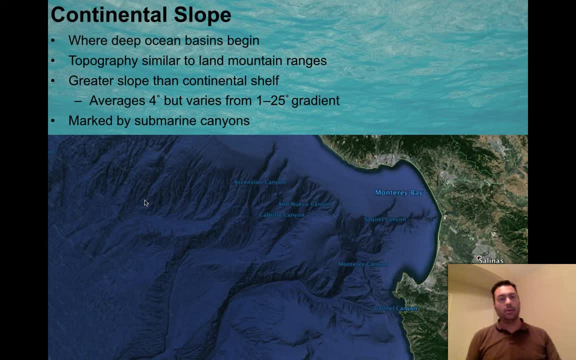 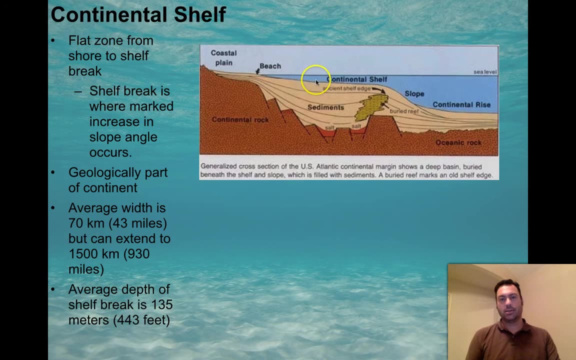 For example, the Grand Canyon or something like this. It has a greater slope than the continental shelf, So remember the shelf. Let's go back to this image. Notice it has a nice slope right here, But it's pretty shallow And all of a sudden, once we hit the continental slope, it drops off. 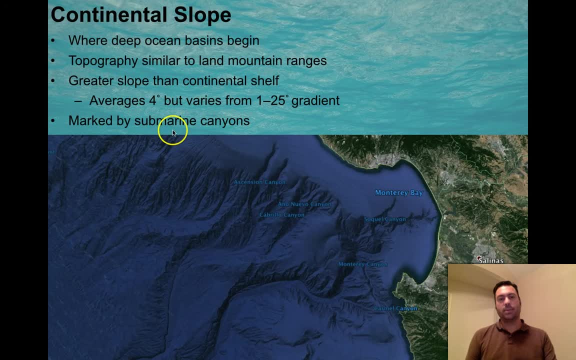 That's all it's saying, And it's marked by submarine canyons. So here we see some really great features. The biggest feature that we see here is Monterey Canyon. This is off of the coast of Monterey Bay in California. This canyon, which is cut into in this place, the continental shelf, and into the slope, is bigger than the Grand Canyon up on land. 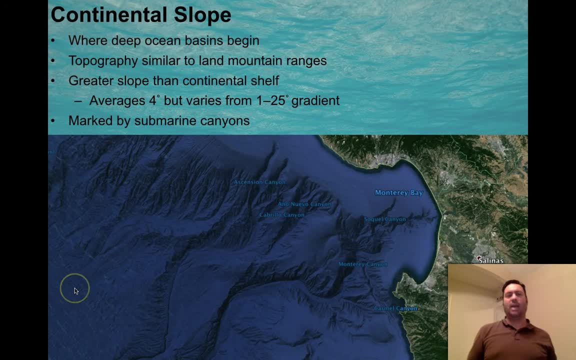 This is a huge feature. How do we get submarine canyons? How do we get canyons that are forming on land? We know that rivers make canyons on the earth, up on the surface. How do you get canyons down below? 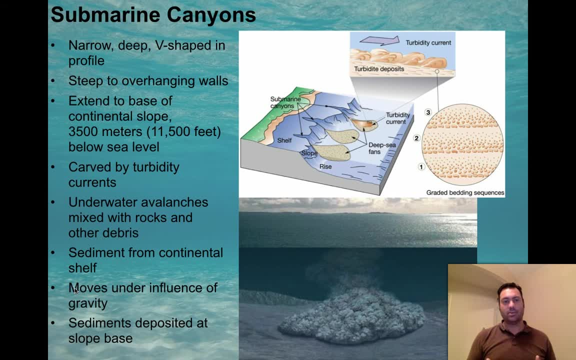 The answer wasn't really easily discovered, But we did finally figure it out. It took a lot of elbow grease. It's taken some time to do some experiments And we were able to figure it out finally. It's very difficult to observe the process. 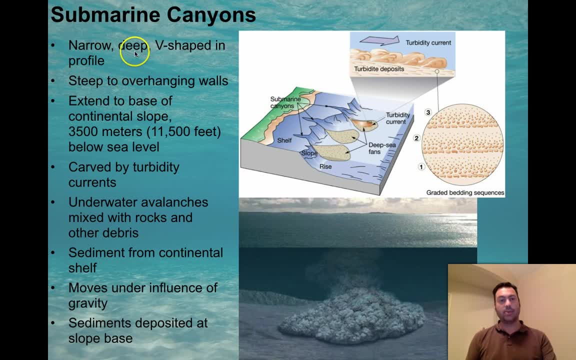 But essentially we discovered that the submarine canyons through mapping were narrow. they were deep and they were V-shaped in profile, The same way that a river is, So it looks like a river Frequently. the walls to these valleys were steep to overhanging. 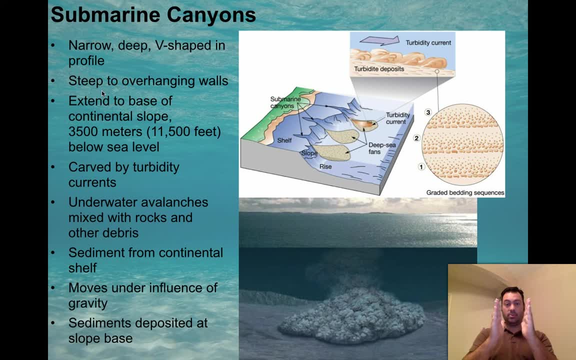 In other words, sometimes they were straight up and down, In some cases even, like this, were held over into the water, And we also found that frequently these canyons extend to base of the continental slope. It means these things reached quite deep. 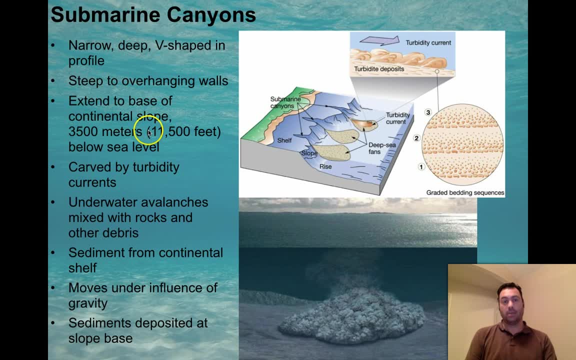 They were long and they were very, very, very deep canyons- 11,000, about two miles deep in some cases, And we have since discovered that they are carved by what we call turbidity currents, which are just simply underwater avalanches mixed with rocks and other debris. 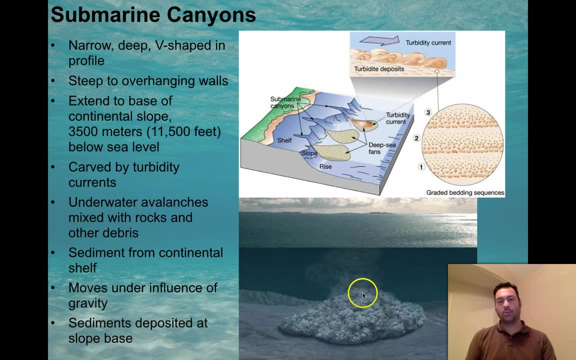 This is a image that was created by an artist showing what he thinks one of these underwater avalanches would look like. So here we see this rock and sand basically moving along the bottom of the seafloor And it's scouring out, almost like a sandblaster, a huge amount of material and digging these canyons deeper and deeper over time. 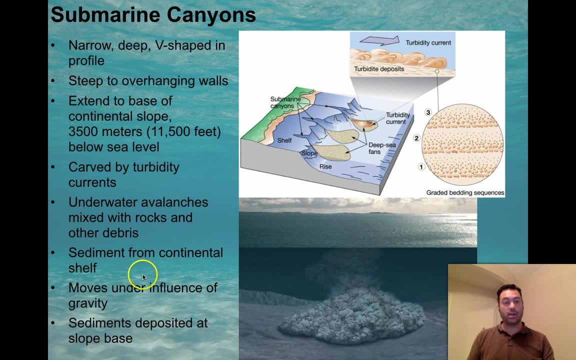 That all the sediment was really just derived from the continental shelf And it's completely moving by gravity. That's what's cutting down these canyons And eventually it forms big lobes at the base of the slope. So that's what this image here is trying to tell us is that we have these canyons. 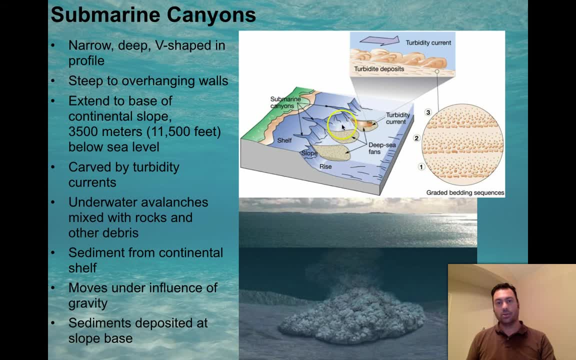 The canyons wind up depositing these large lobes of sediment And we, in the process of making them, we occasionally come in and create turbidity currents. These turbidity currents, by the way, when they settle out in the water, have a pretty distinctive graded bedding sequence that we can recognize. 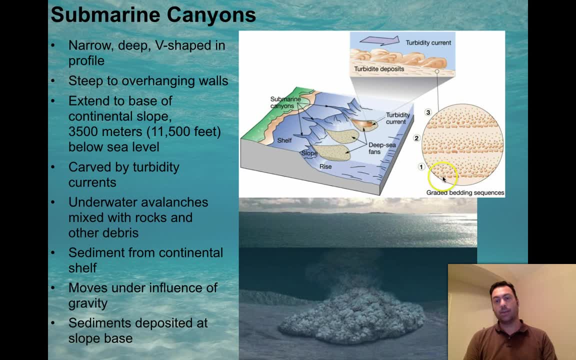 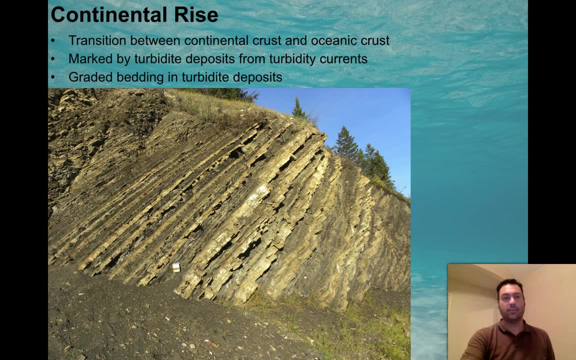 As geologists, where it gets really coarse at the bottom and it gets fine at the top, And then it repeats. every single time one of these happens, And we find it all over the Earth. In fact, here's one right here. These are nice slope deposits. 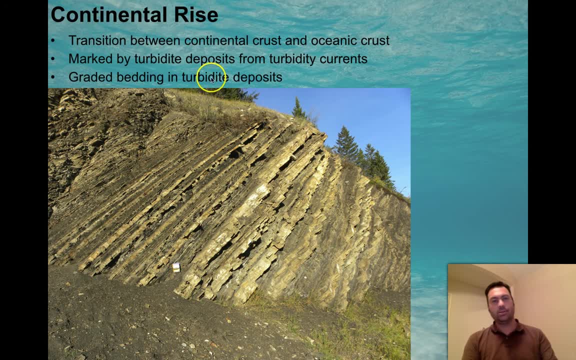 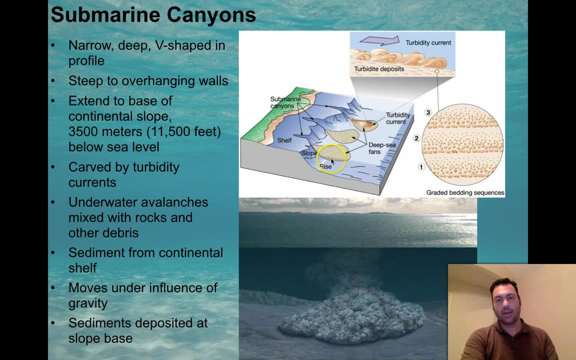 And even right out onto the continental rise, rise deposits, And this is the transition between the continental crust and the oceanic crust. This is where these things start getting piled up. So let's go back over here. Here's the rise And these are where these lobes of material are. 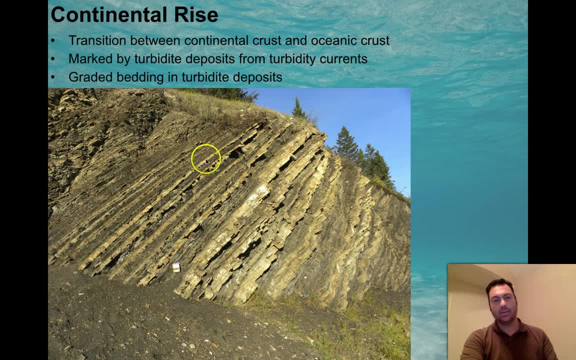 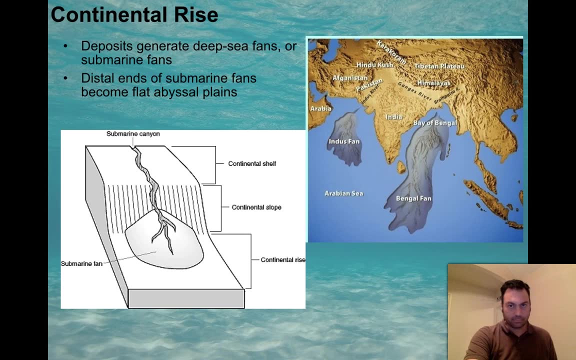 All right, And so here we see those rocks as they're being formed in the deep ocean, In this case up on land. The continental rise has some really neat features. We were talking about how you have these submarine canyons that wind up moving a large amount of sediment out into the open ocean. 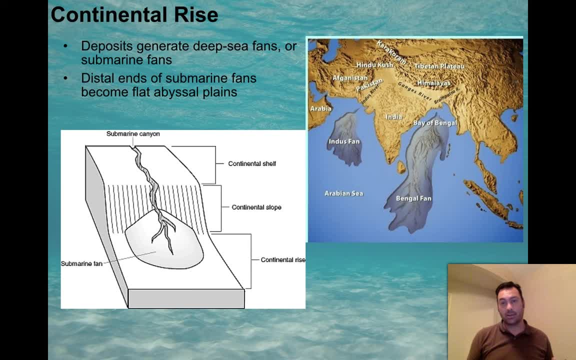 But when it gets out to the open ocean, out onto the sea floor, it piles up Right. It doesn't continue as a river across the oceans, It actually piles up right there at the bottom of the channel of the submarine canyon, And so the distal ends of submarine fans become flat, abyssal plains. 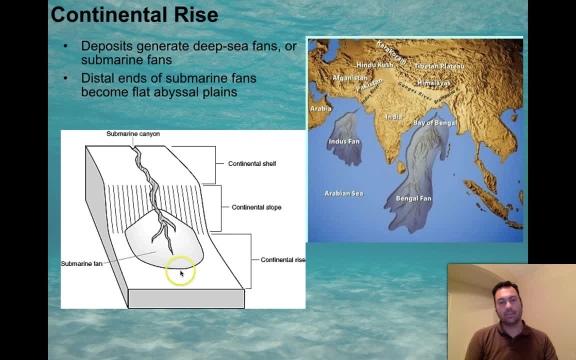 So we wind up with a pile of it here. The distal means the farthest part right out here And then out here, where we're not able to pile up any sand or any of the rocks that are coming through the submarine canyon. it's pretty flat. 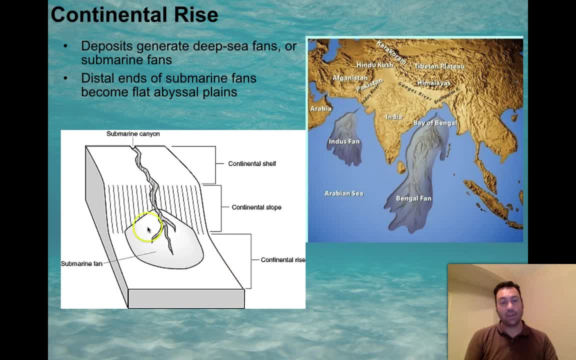 That's what that is basically. That's what that is basically telling us. Now, these features, these big submarine fans, and that's what these things are called. these big piles the bottom of the continental slope can get huge. When we look into the Indian Ocean, we find that there's a huge fan called the Indus Fan that is being deposited by the Indus River. 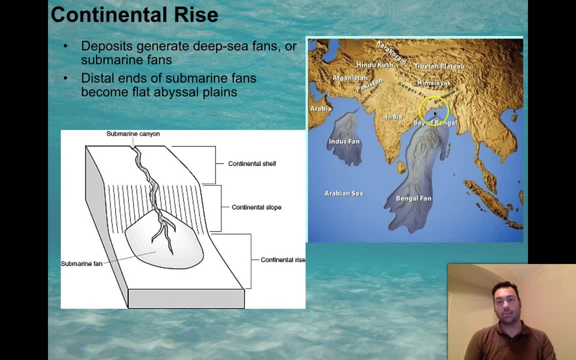 The Bengal Fan has the Ganges and the Brahmaputra And those rivers are dumping into the Bay of Bengal And the Bengal Fan is the largest pile of sediment on planet Earth as it exists today And you can see, this pile of sediment is longer than the nation of India. 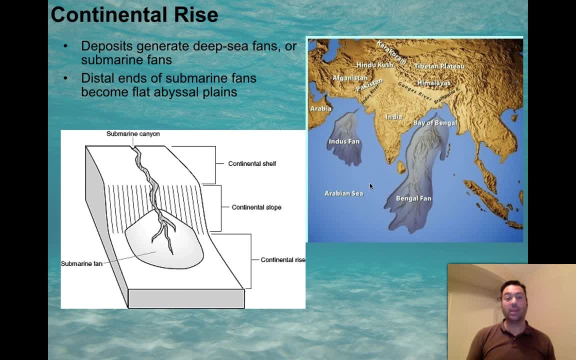 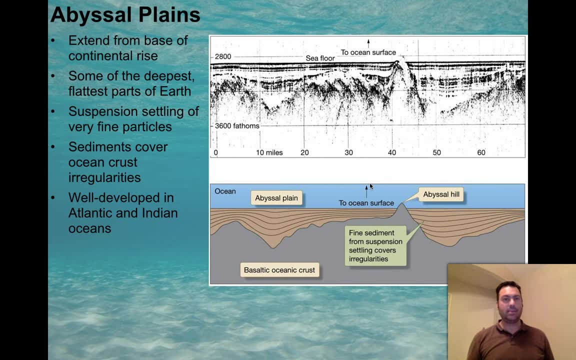 This is the nation of India right here. This is a really really cool feature. Now, once we get past those big piles of sediment, we get into the abyssal plains- Really flat surfaces. Now that doesn't mean that the bedrock is flat, but there's some really interesting things that happen. 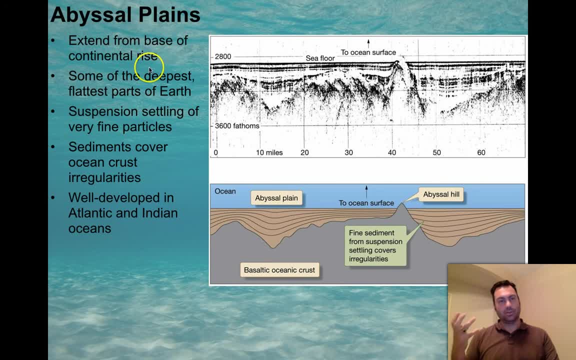 So these extend from the base of the continental rise. That's where those lobes of sediment are, And some of the deepest, flattest places on Earth. It's basically like an open, wide, plain, Suspension settling of very fine particles. In other words, a lot of very, very small stuff settles through the ocean and out into the nice, calm water of the open ocean, into these abyssal plains. 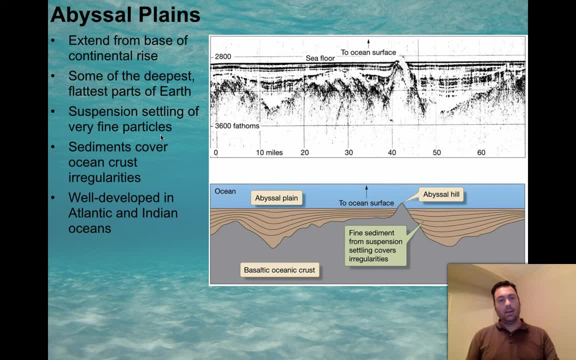 And so you get a lot of clays there, And the sediments tend to cover ocean crust irregularities. So here, this might be what the ocean crust formed when it was volcanic and active and young, But since then the holes have all been piled up and filled in. 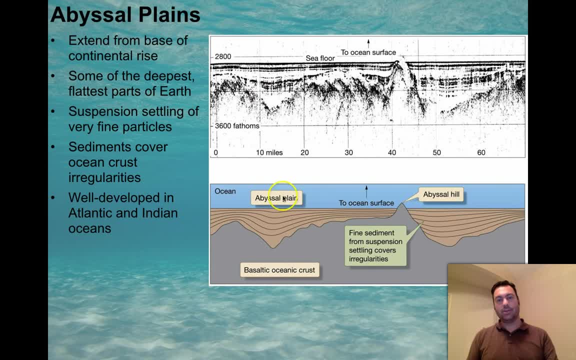 And we get a nice flat surface. In fact, this is an interpretation of this image. Notice the word fathoms here. So if you multiply that number by 6, you get the number of feet to the depth of that seafloor. 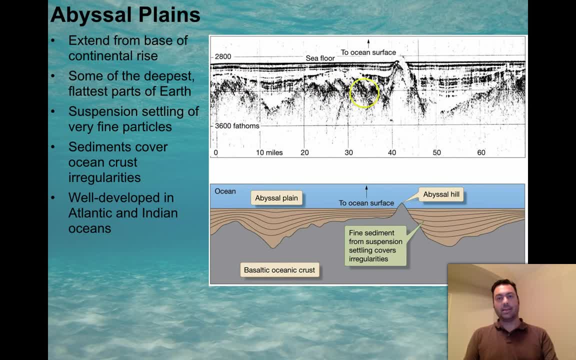 And we can see. here's the bedrock. The bedrock is not even at all, But the sediments have come in and filled in these nice layers all throughout here and made it into a nice flat plain, And so these plains are actually pretty well developed in the Atlantic and Indian Oceans. 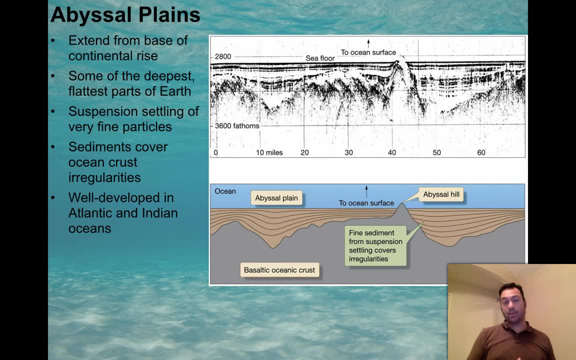 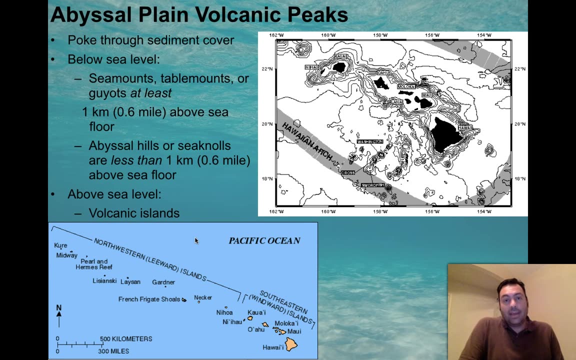 There are some abyssal plains in the Pacific, But there's problems that are happening out there that are preventing the development of this type of perfect plain, And we'll be coming to what those are in a future lecture. Okay, So the abyssal plain tends to have some really neat stuff going on. 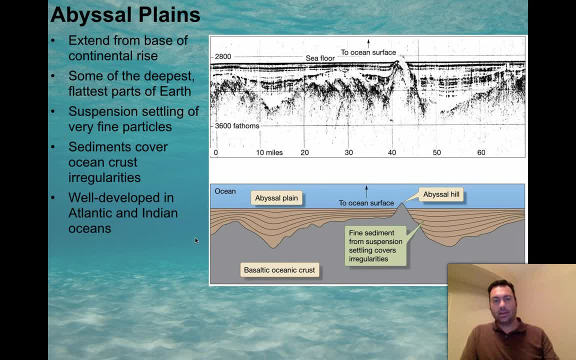 Let's go. actually I got a little ahead of myself. Look at this picture right here. Here we see an image of a hill sticking up out of the sediment right. But when we look at the profile here, we notice that the hill is actually coming up out of the sediment. 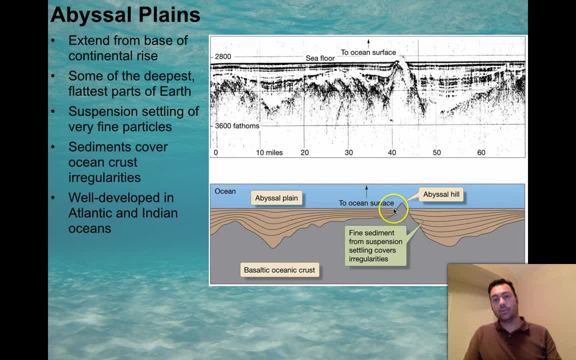 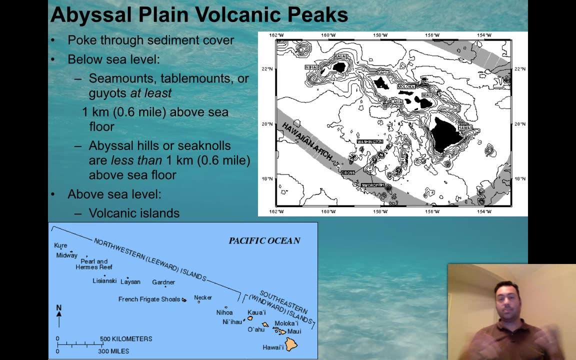 But it's a much bigger hill than what we would see on the surface. The surface only shows this amount, But the actual bedrock goes quite deep, And so before this was covered, it was quite a tall hill. Okay, So there's a lot of topography that's constantly getting covered over. 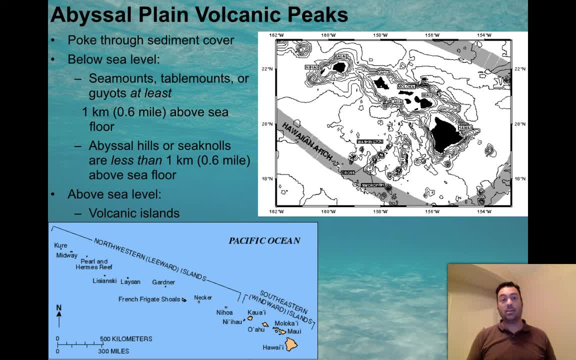 However, there are some things that even the abyssal plains can't cover up. Okay, And we get things poking through the sedimentary cover. They're called volcanic peaks, Abyssal plains, Abyssal plain, volcanic peaks. The classic example of these are the Hawaiian Islands. 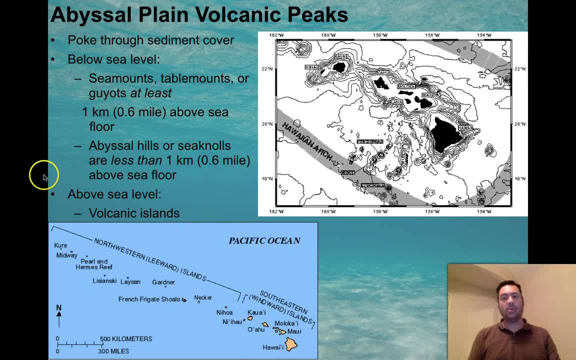 Okay, So any volcano that is forming on the bottom of the seafloor that's poking through, these are called seamounts. Sometimes they're called table mounts- We'll talk about the evolution of these a little bit later- And these have to be about a kilometer above the seafloor. 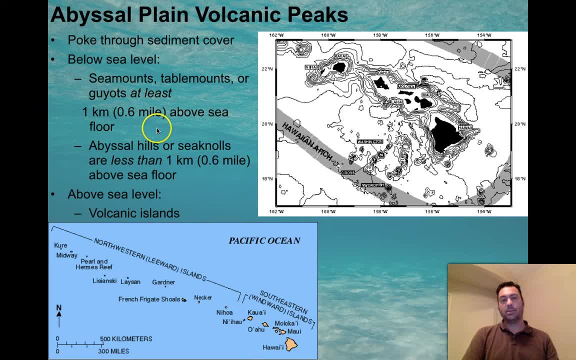 They're pretty tall, They're really big, They're not abyssal hills which are less than a kilometer high. Okay, Anything above sea level is a volcanic island by definition. So in this case, the seamount has poked its way out, all the way out of the ocean, out of the water. 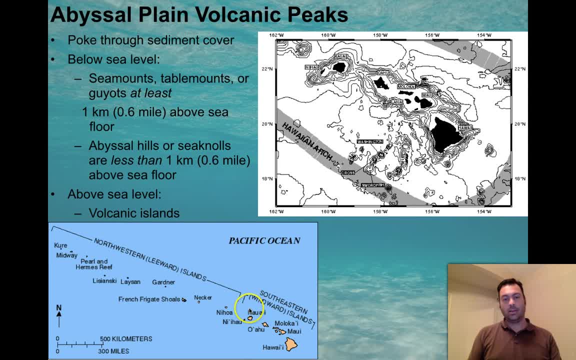 In Hawaii. we see the state of Hawaii located right over here, the principal islands, the big island of Hawaii, Oahu, and so on and so forth. But as we trail off in a single direction, we talked about plate tectonics, about how the plate is moving. 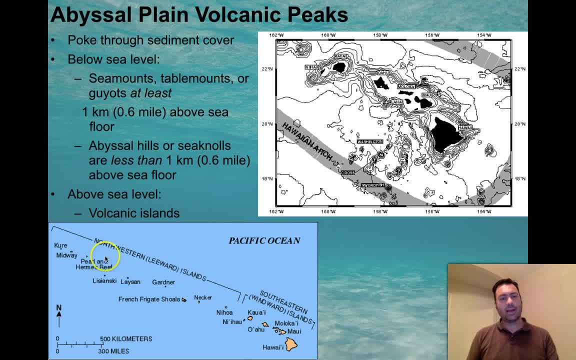 It leaves behind a series of volcanic islands and eventually seamounts, And these seamounts are all over the place Now. when we just look at the surface, we don't actually see everything that's going on. So let's come to this image here. 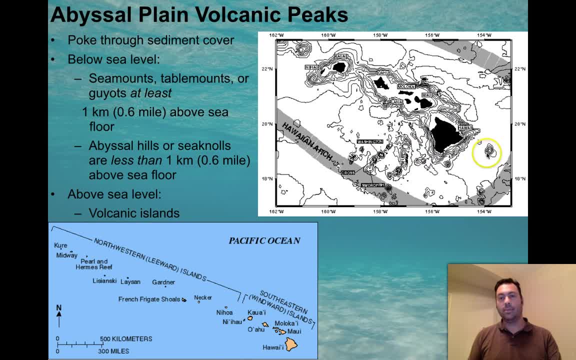 This is a bathymetric map. Here we see the big island of Hawaii And there's a seamount. There's a seamount, A whole bunch of seamounts located in here. Another seamount- here You get the idea. 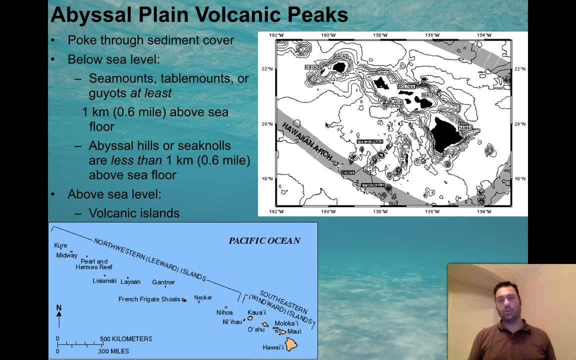 It turns out, there's a lot more going on underneath the water. There's a lot more going on underneath the water around Hawaii than just simply the islands that we see. There's basically low-level islands that just haven't made their way out either yet, or if they had, they'd eroded down. 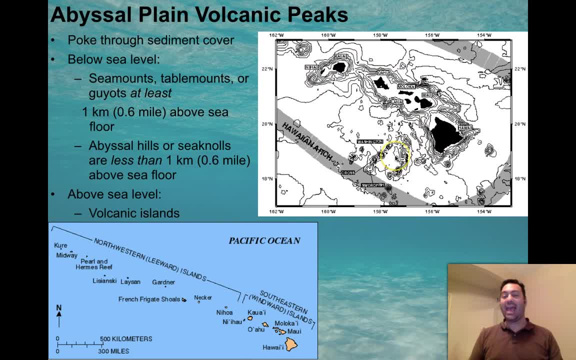 And there's a tremendous amount of gravitational weight added by the formation of Hawaiian islands in that area And it causes the crust there to bow down a little bit. So it creates something called the Hawaiian arch, which is the bowing down of the crust at that location. 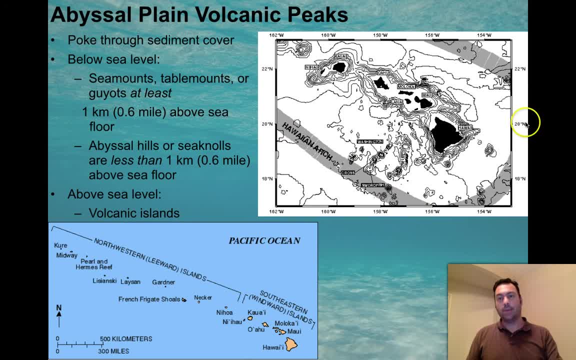 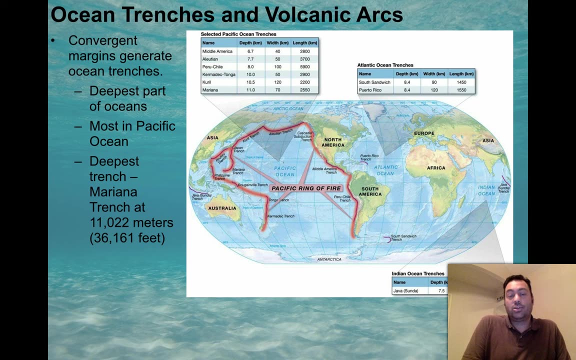 And so this bowing down usually occurs, according to this map, within this gray zone. So this is all sitting lower than the rest of the ocean out here. Kind of neat. So there's some geomorphic features that are associated with certain provinces. 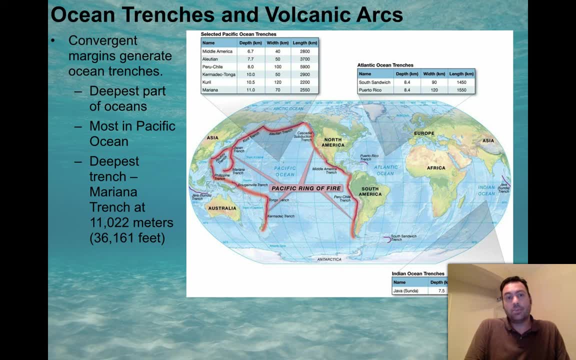 Ocean trenches and volcanic arcs, for example. So convergent margins- let's go back to that again. They tend to generate ocean trenches. We brought that up early on. Let's come back to that a little bit. So what is an ocean trench? 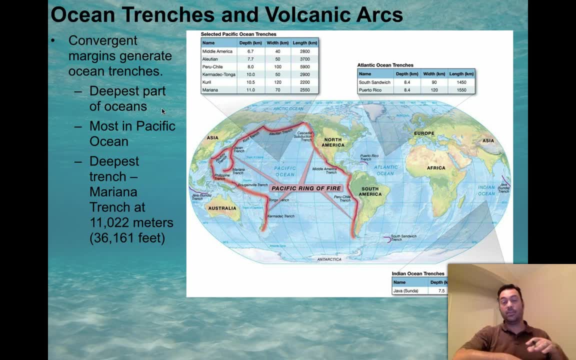 Well, they're places where the subduction is happening, And if it's a vigorous area, you can get very deep depths as it's going down into that trench. Most of them are in the Pacific Ocean. In fact, the deepest trench, the Mariana Trench, is 36,161 feet deep. 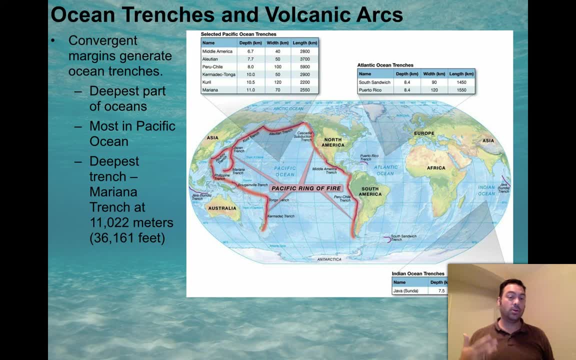 That's deeper than Mount Everest is tall. So, as a matter of fact, it's over a mile higher than Mount Everest is tall. So you can put Mount Everest into the Mariana Trench and there would still be another mile of water sitting on top of it. 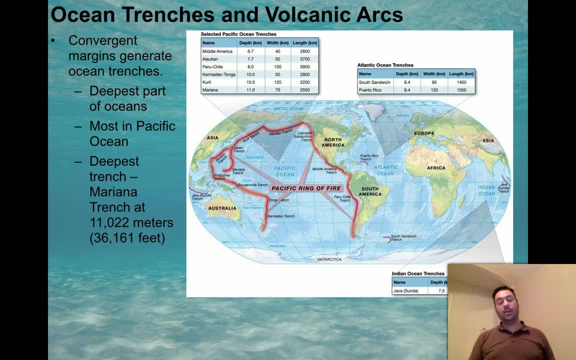 That is a tremendous amount of relief, A tremendous feature at the bottom of the ocean for which we can't see. And where is this located at? Is it right in the middle of the ocean out here? No, In fact, right out here in the middle of the ocean. we're pretty close to the Hawaiian Islands, which, as we know, are sticking out of the water. 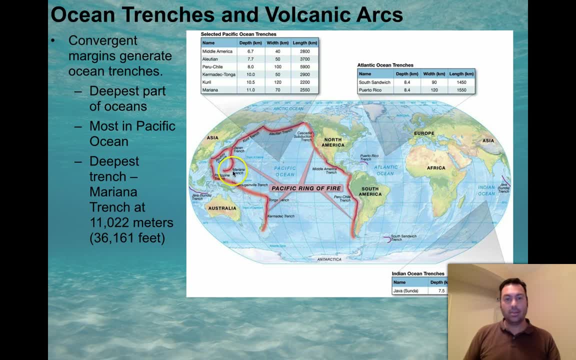 So it's not very deep right where the Big Island of Hawaii is. The Mariana Trench is located right over here, way over here on the western part, And so this was again another confirmation of plate tectonics. If you haven't seen the video on plate tectonics, please pause right now and go and watch that video and then return to this one. 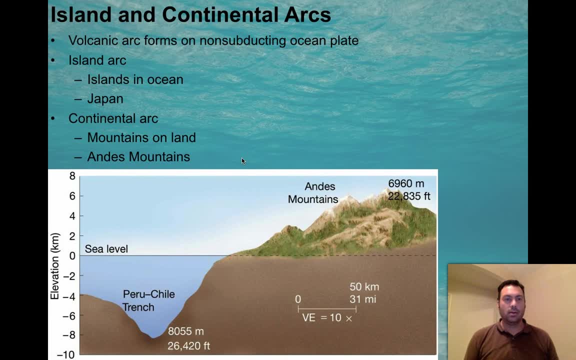 All right, And so this is what we see in terms of the bathymetry of island and continental arcs. So the volcanic arc forms on non-subducting oceans. So we get the volcanoes forming over here. We wind up with the Pacific Plate. 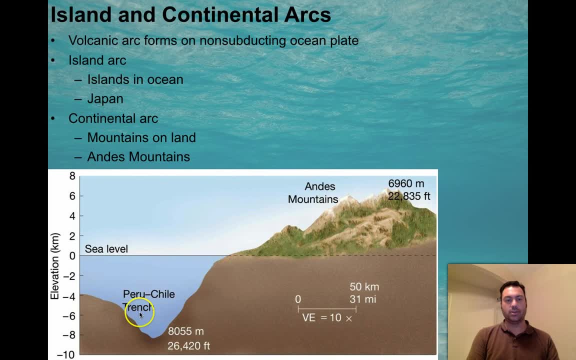 In this case, this is going to be the Andes Mountains, the Peru-Chile Trench of South America, And it's subducting beneath here and creating these volcanoes, But we wind up with this deep trench right next to these really high heights. 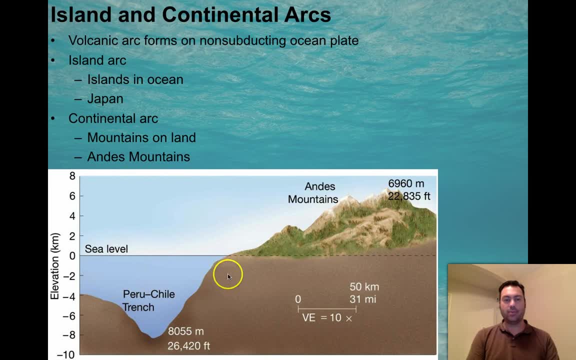 It's really cool that we can get that much relief. We go from 26,000 feet deep to 22,835 feet high And really only about 150 kilometers, or maybe 200 kilometers if we use the scale here. Okay, That's a tremendous amount of relief. 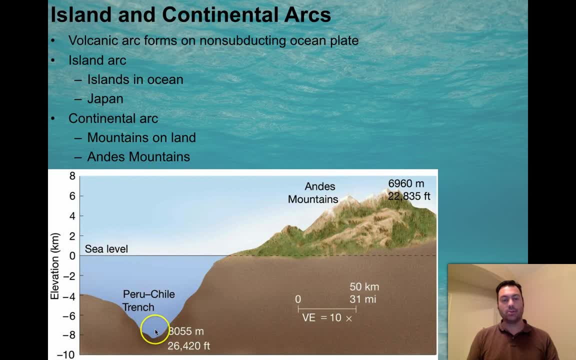 So if we drain the oceans and we started walking- so this is a drained ocean- we start walking up this right. that's five miles up to just the beach and then another four and a half miles to get to the top. That's almost ten miles of relief just at one of these island and continental arcs. 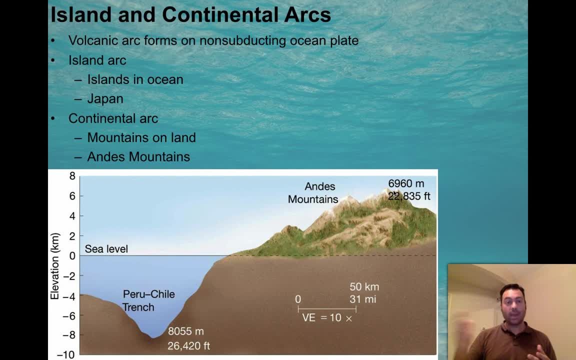 Just at one of these island and continental arc locations, like what we see in South America. This is a really cool place. These happen a lot in the Pacific Ocean: the islands and the ocean. Japan is a classic example Continental arc and this would be in the case of an island arc. 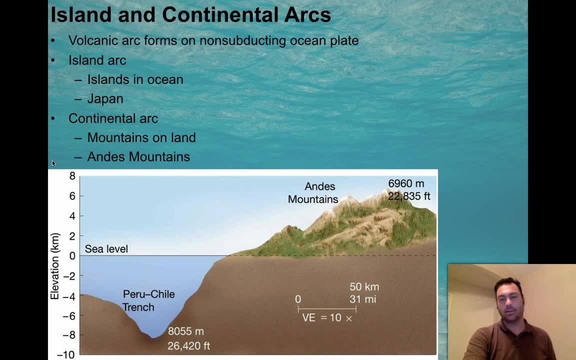 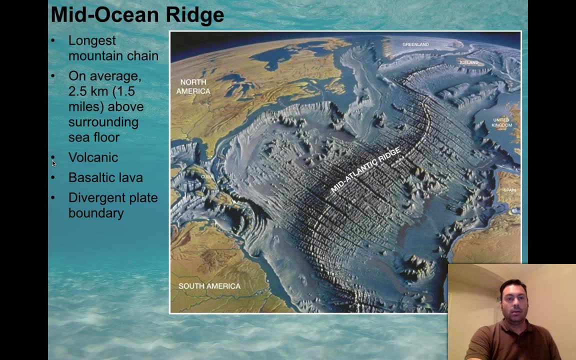 But in the case of a continental arc, the Andes Mountains of South America are a good example, as well as the Cascade Mountains of northwestern United States. The Mid-Ocean Ridge is the longest mountain chain. Here we see the Mid-Atlantic Ridge. 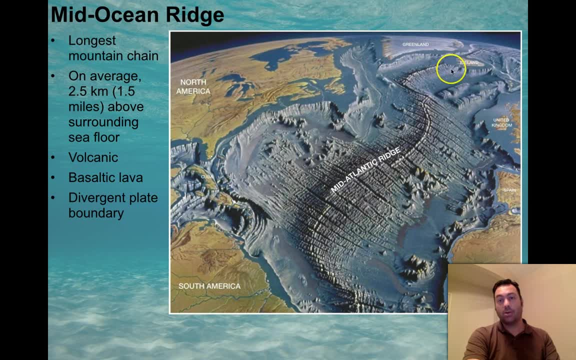 This extends all the way through Iceland. Iceland is, in fact, a part of that ridge where it sticks up out of the water, And this extends all the way down towards Antarctica. On average, it's one and a half miles high above the surrounding seafloor. 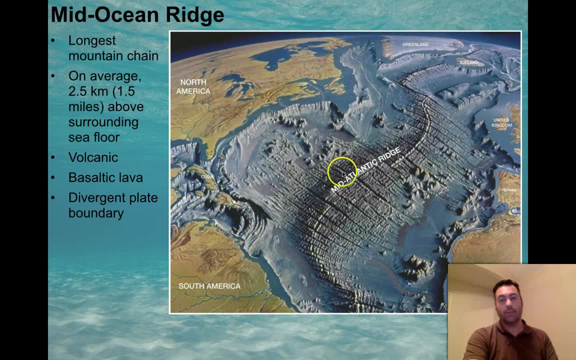 So it's a pretty tall feature. Notice it's also quite wide right. This extends about a third of the way between Africa and North America. Here we can see the continental shelf, The slope and the abyssal plain. They're volcanic. 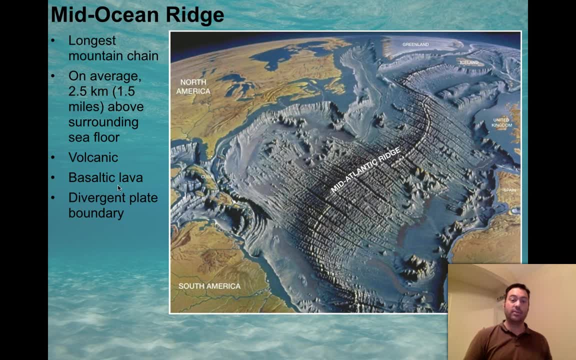 Lots of volcanism that's happening here, A lot of basaltic lava, Black rock right And a divergent plate boundary. In other words, the rocks on this side are moving in this direction. The rocks on this side are moving in this direction. 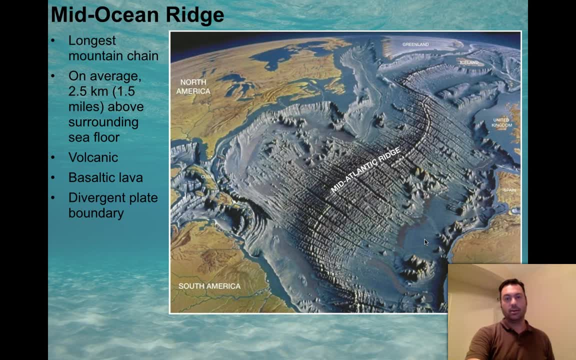 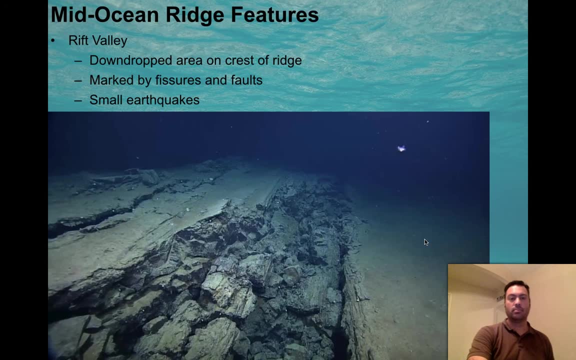 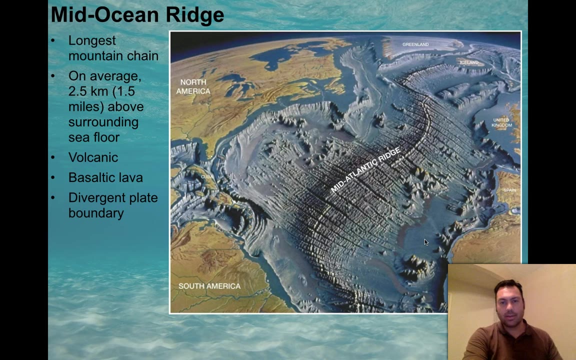 They're moving away from each other. Divergence is happening here By comparison with convergence in the case of forming of a trench. We've gotten video of these things. We've got lots of pictures And we find that right at the top and we can see these things. 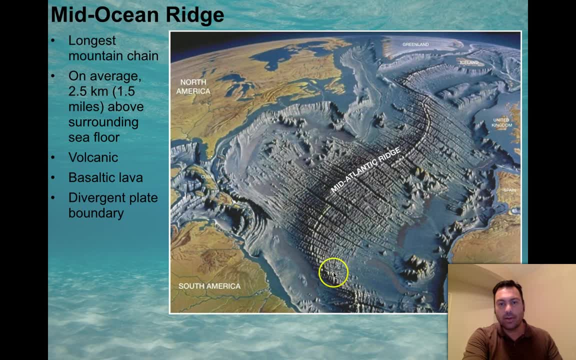 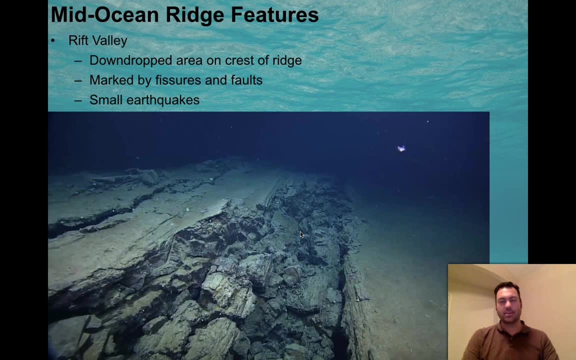 You can see that there's kind of a rift valley located right here. We've gotten in and we've gotten photos of them. Here's a rift valley In this case. this is a rift valley, I believe, in the Pacific, in the Southeast Pacific. 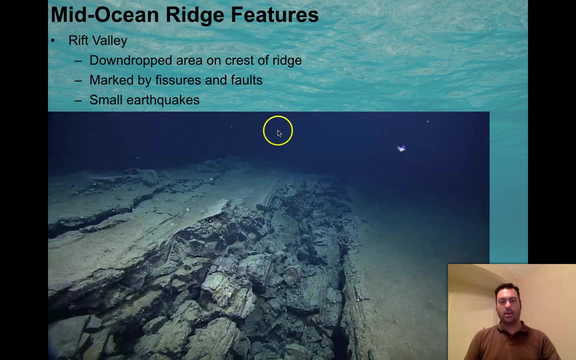 And here we see that, as it's pulled apart, this portion of the rock has dropped down. It's making that big rift And it's dropping down the center part of it as the whole region pulls apart. It's marked by fissures and faults and lots of very small earthquakes. 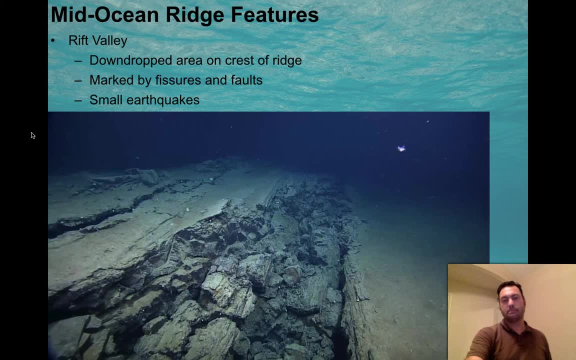 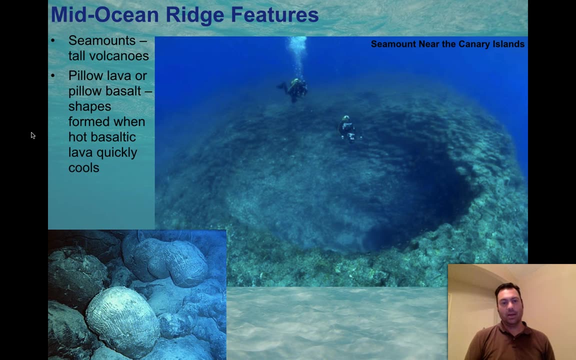 Thousands and thousands of small earthquakes. Another really cool feature about these things are the seamounts. These are usually very difficult to study because unless a satellite tells you that it's there, you don't know to go there. There might not be any supply nearby. 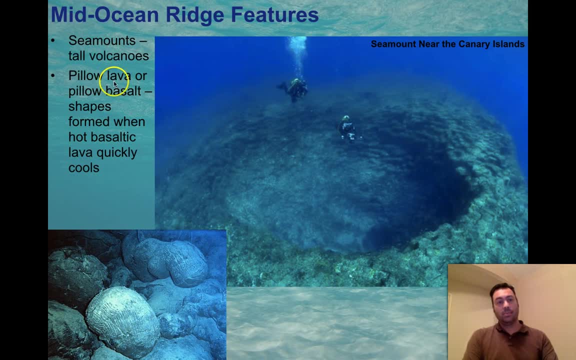 And so they're really poorly studied. But seamounts are just really tall volcanoes on the seafloor, That's all they are. Here we see a couple of divers that are exploring a seamount that is near the Canary Islands, which is off the coast of Africa. 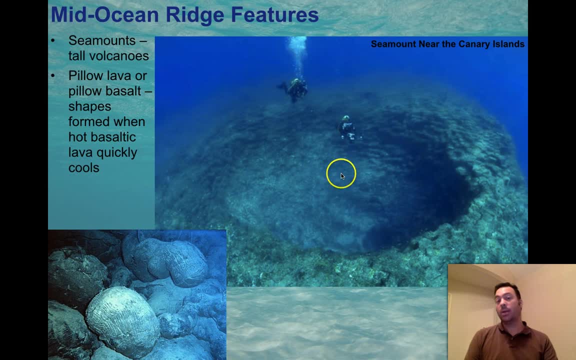 They're just lucky enough to be in an area where they're able to look at a volcano that is very, very close to the surface of the ocean, So close to the surface that light is actually able to see it, It's able to penetrate and to show us that the volcano exists. 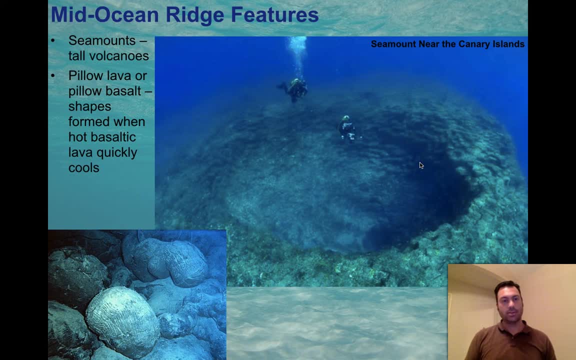 If it was any deeper, you wouldn't even be able to see it. You'd have to take special cameras to see it. One of the things that these things form is a type of basaltic lava called pillow basalts, And instead of flowing out almost like a river, flowing all over the hillside, like what we would see at Kilauea. 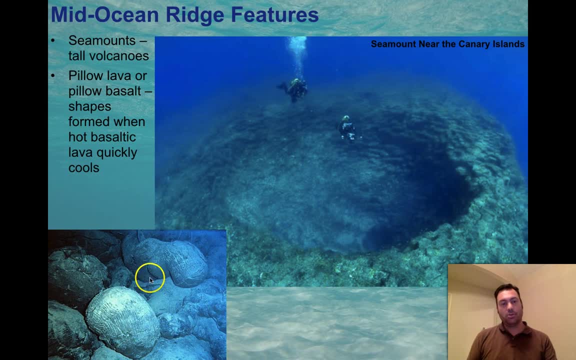 as they flow underwater, it forms these big bulbous blobs called pillow basalts, And here we can see the pillows in the sides of this volcano. here These are pillow basalts and this is them up close. And this is actually pictures of pillow basalts off the coast of Kauai. 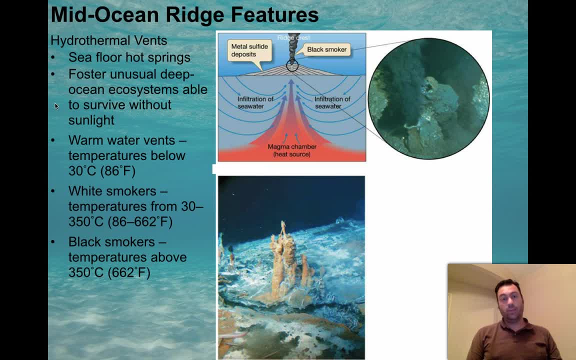 So there's also some other really cool ridge features that we need to bring up because they're going to become really relevant as we move forward in the class, especially when we start talking about life and the origins of life in the oceans At the mid-ocean ridges, because they're volcanic- there's also hot springs in the area. 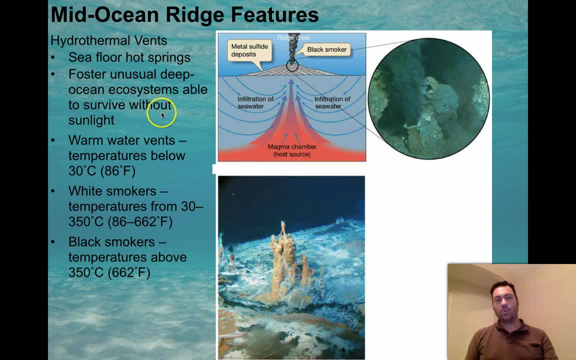 seafloor hot springs all over the place And these wind up fostering all kinds of unusual ocean systems, right ecosystems. The reason why they're unusual is because sunlight has not penetrated into this area. It's so deep that there's no light in the area. 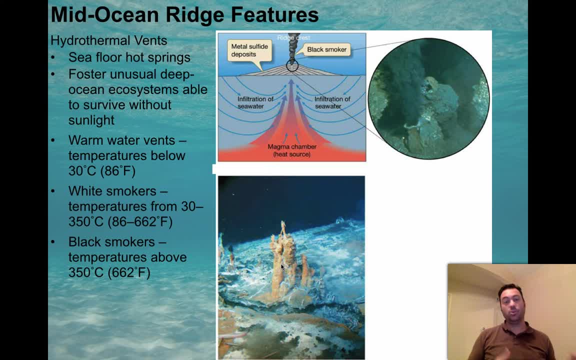 So we don't get photosynthesis of plants, We get unusual animals that live in this area. So how do they live, you might be asking. Well, it turns out that the water in the ocean, the warm water vents, provide them with everything they need. 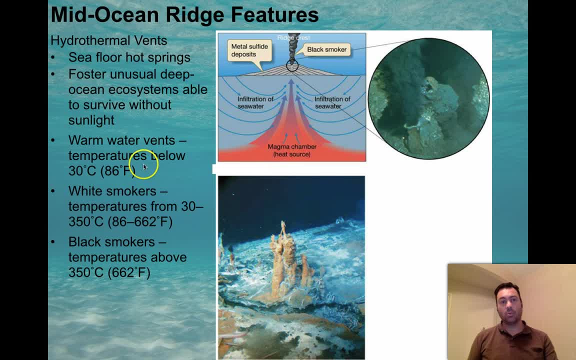 The water is about 86 degrees Fahrenheit. in the case of the warm water vents, You can get white smokers. White smokers produce a lot of mineralization of the water, providing nutrients and chemicals, But the temperatures can get much hotter than just the warm water vents. 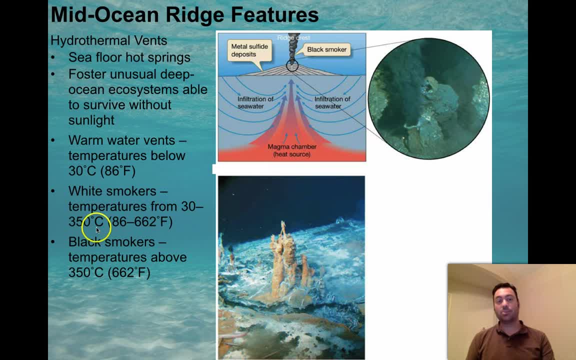 It can get between 30 and 350 degrees Celsius. That's three times hotter than boiling, Three and a half times hotter than boiling. And the reason they can get that hot without actually boiling the water is because the pressure is so high that it prevents the boiling from happening. 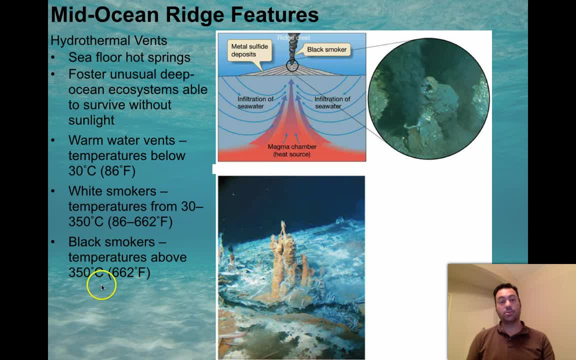 Black smokers, those can get at temperatures above 350 degrees Celsius. In fact, here's a picture of a black smoker with minerals coming out of this seafloor hot spring And, believe it or not, there's life in that area that can survive in the presence of such a hot water presence. 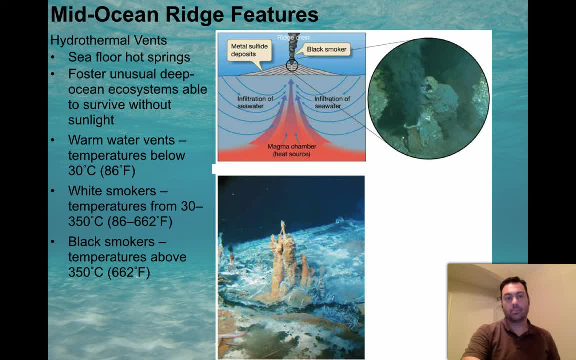 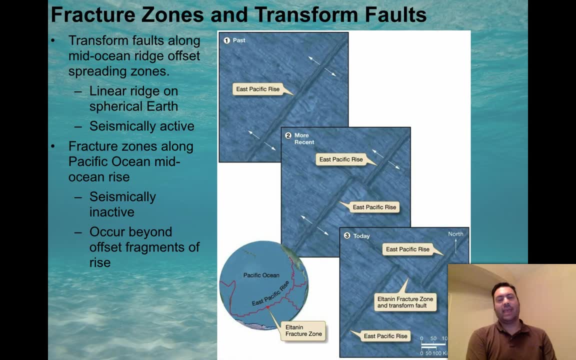 Now, when we look at the maps, we discover pretty rapidly that you can't have a rift zone going through the middle of a, you know, kind of an S-shaped Atlantic Ocean without having troubles, right, Because the rift zone is a nice straight plain. 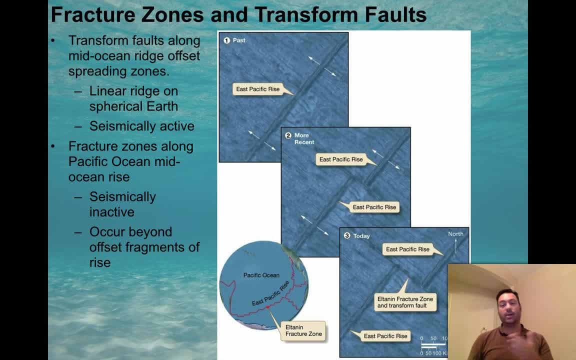 The Atlantic Ocean forms an S, And so how do you move that around over time and get it to bend in different directions? The answer is: is that the faults themselves? that ridge is cut by other faults, It's faulted. Okay, so transform faults are what we use to do this with. 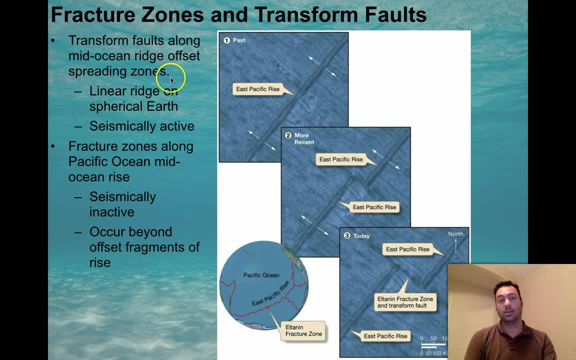 And so transform faults along the mid-ocean ridge, offset spreading zones. So here we see a spreading center right here, say, the East Pacific Rise, And what you can do is you can cut a linear ridge on the spherical Earth, or I'm sorry. 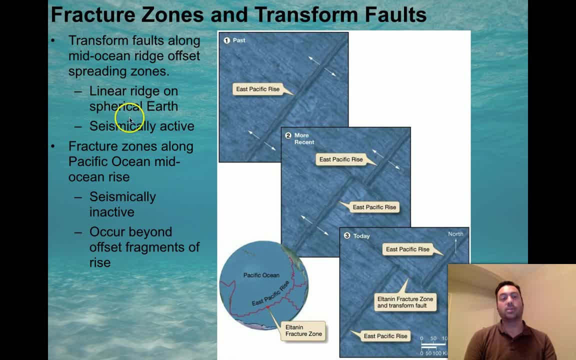 I'm getting ahead of myself. It's a linear ridge on the spherical Earth, seismically active. Sorry about that. What I mean to say over here is the fracture zones along the mid-ocean ridges and specifically the Pacific Ocean. 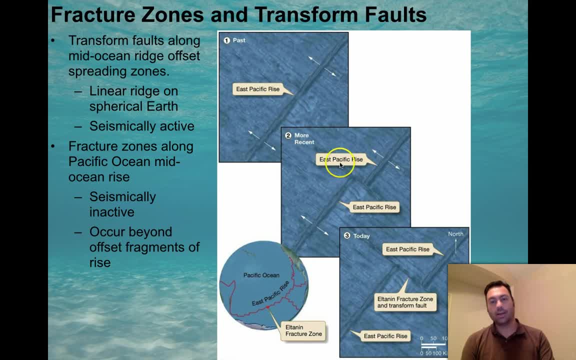 mid-ocean rise is. you can actually cut, using a transform fault, this spreading center and offset it. So this and this are moving, but notice that this then jumps over and moves like so, And over time that can expand. This will be moving and this will be moving. 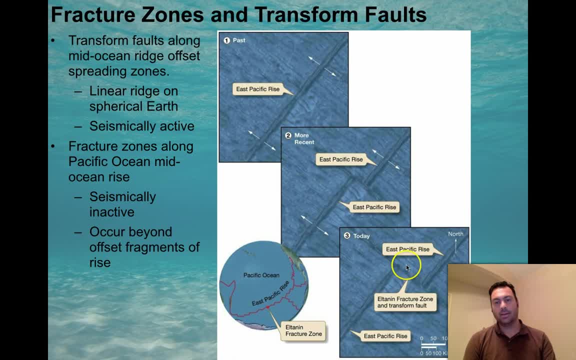 but this fault right here is now not spreading. it's actually sliding past right, Because the rocks right here are going this direction and the rocks right here are going this direction. So this is a shear stress, whereas these are normal stresses. 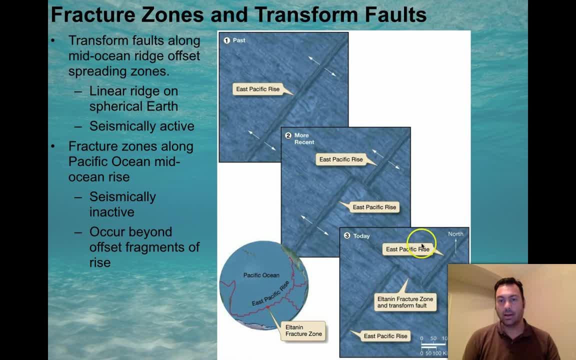 or which is to say, tensional stresses across the rise. Okay, So it's just a way of being able to move the motion around so that we can move things around. So here we see, on this, this globe, here, here's the East Pacific rise. 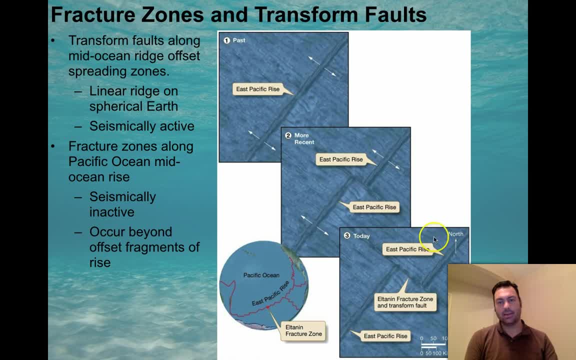 and we see that it's kind of zippered in, and it's zippered in along these transform faults. So where are the earthquakes going to happen? They're going to happen from here to here Out here. is there anything happening? Nope. 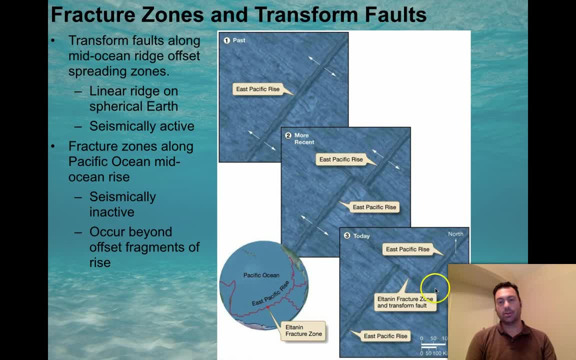 Right, Because the rocks here and the rocks here are both going the same direction. The rocks here and the rocks here are both going the same direction. These are both going to the southeast, these are both going to the northwest, so they're fine. 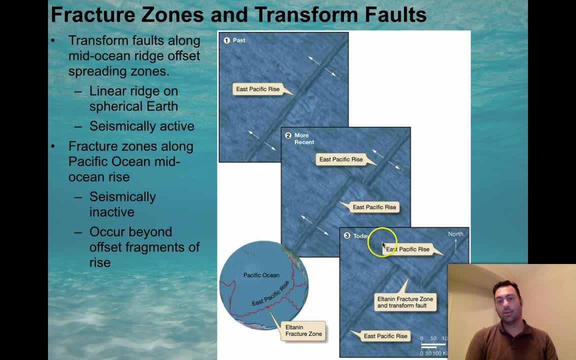 There's not going to be any earthquakes, But here they're going to the northwest and here they're going to the southeast. there's going to be earthquakes right along here. So this is a seismically active zone right here, And so what would this look like in cross-section? 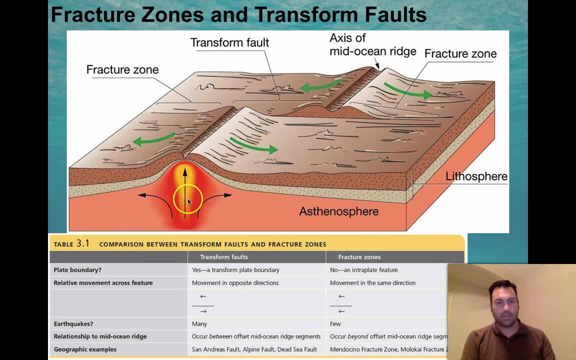 Well, here we have our magma chamber. here we have our spreading in this direction and this direction. Here we see our transform fault that is offsetting the spreading over to here, in this direction and this direction. We have earthquakes that will occur from here to here. 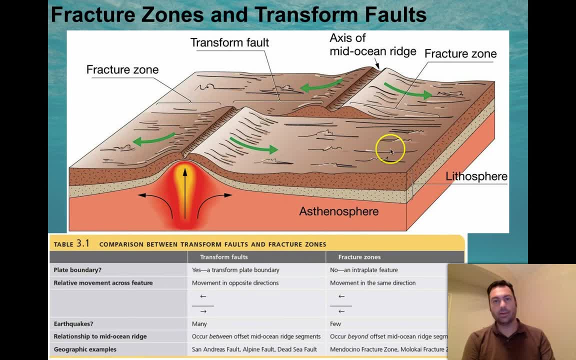 but not from here to here, because, remember, they're both going the same direction. Okay, And this is an image from the textbook I traditionally use in the class that can help you figure out what to expect at any part of a transform fault or the fracture zones that extend beyond that transform. 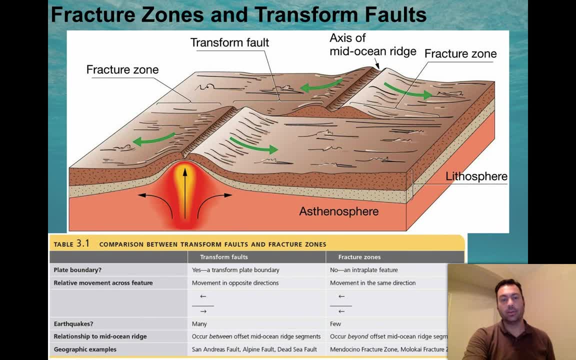 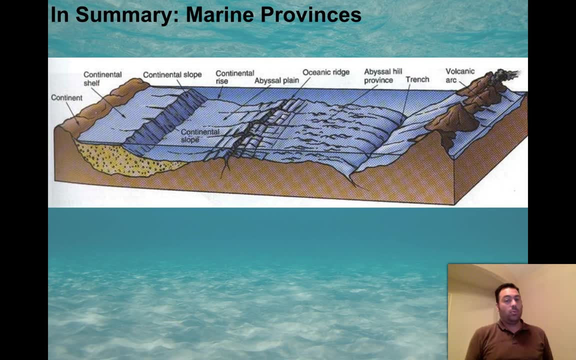 Okay. So if you need to go ahead and pause the video and look at this little table 3.1 that I've included in here, All right. So, in summary, you know we have some dynamic things that are happening on the sea floor that are important to understand. 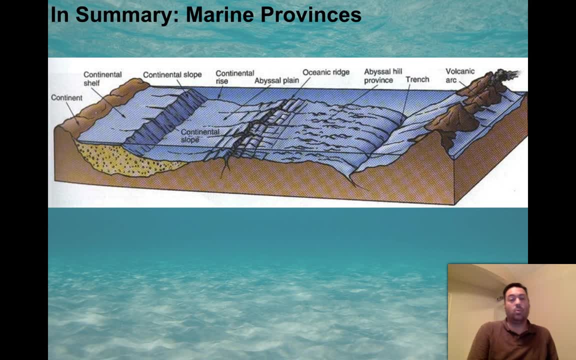 because it has a traumatic effect on the way that we deal with the oceans, how we interpret the oceans, how the animals in the ocean behave, And without understanding the marine provinces, which is to say the mid-ocean ridge, the abyssal plains. 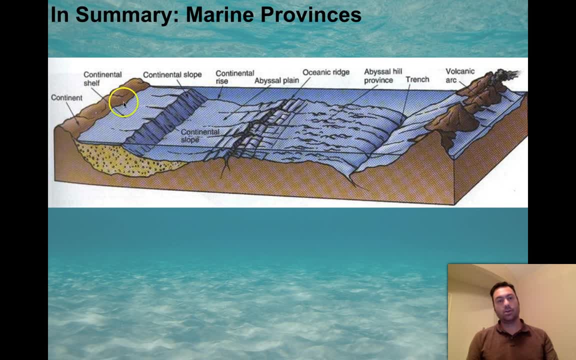 right, the trenches and the volcanic arcs, the continental shelf as well as the continental slopes, all that stuff. we're not really going to have a full understanding of the ocean and the animals that dwell within it, So we're going to be building on this as we go forward in the class. 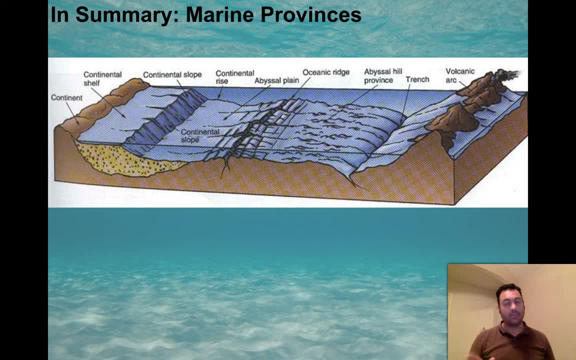 I hope you enjoyed the lecture and you got something out of it. It's kind of a dense lecture- a lot of information, a lot of geology, describing techniques and things like this- and I hope you didn't get lost. So if you have any questions, 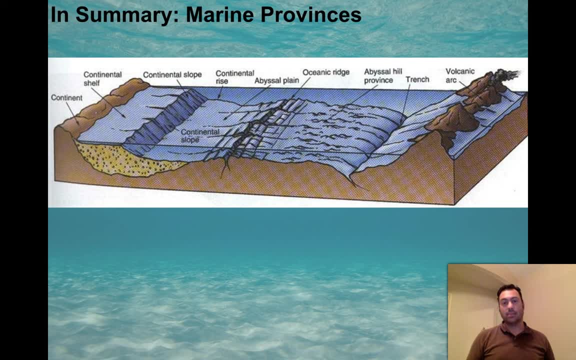 as always, send me an email And until next time, I hope you do well Take care. Bye.